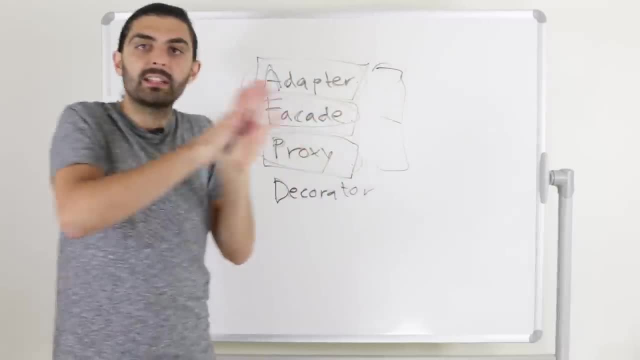 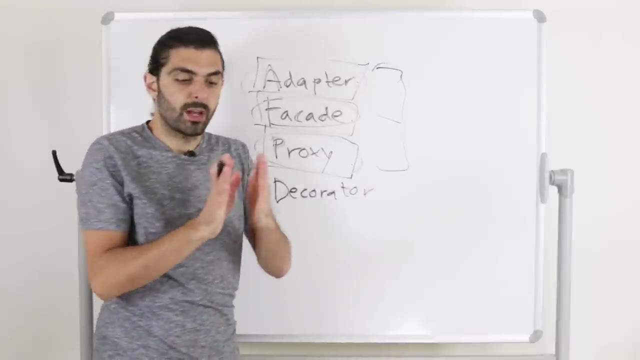 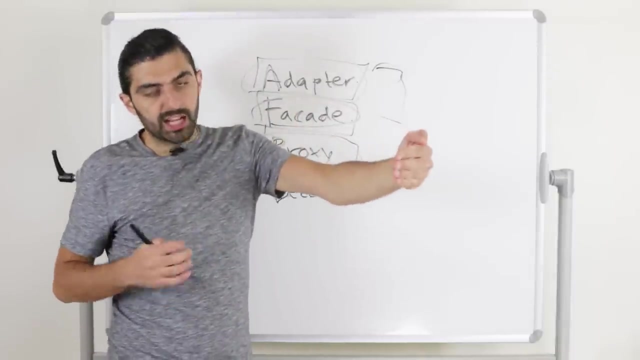 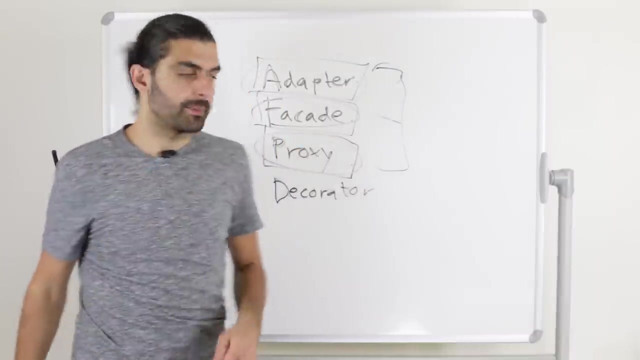 is about taking a bunch of complex interactions and creating a facade that you can use instead of having to deal with all of those complex objects and complex interactions. Proxy is a way of placing a proxy between something that you want to call. So you want to call a particular thing, but instead of calling that thing, you call the proxy. who calls that thing? The reasons could be, for example, security or caching or stuff like that. And finally, decorator- we know from before- is a way of 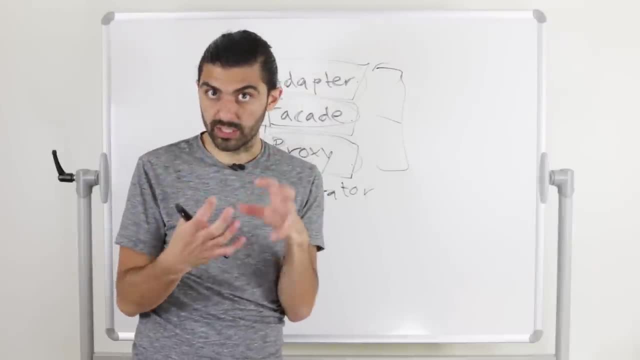 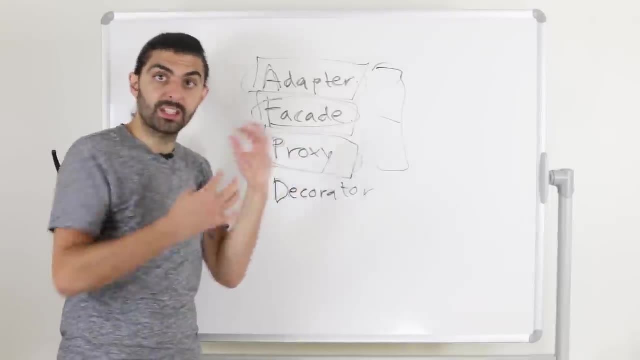 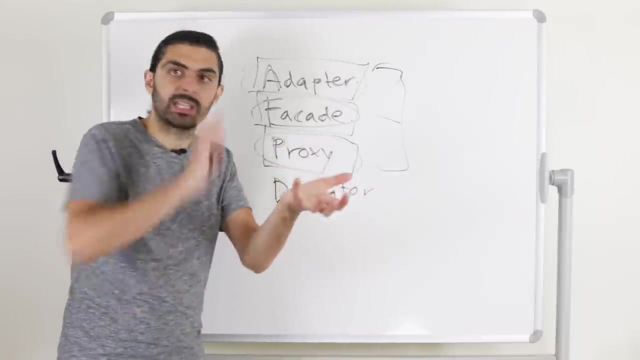 adding behavior to some particular object without actually opening up and changing that object. Adapter makes interfaces compatible, Facade hides some complex logic. Proxy intercepts a call and thus controls access to the underlying object. And decorator adds behavior to some particular object, the object that it's decorating. Now let's forget about all this stuff And let's only talk about 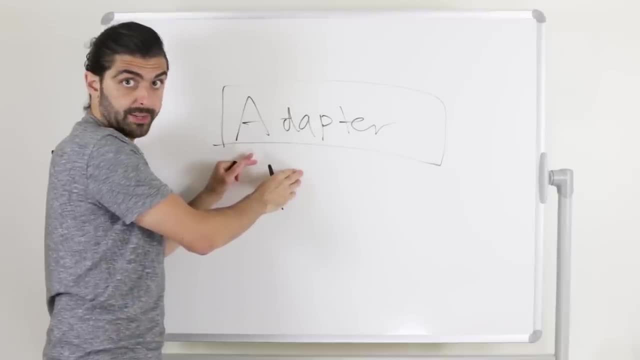 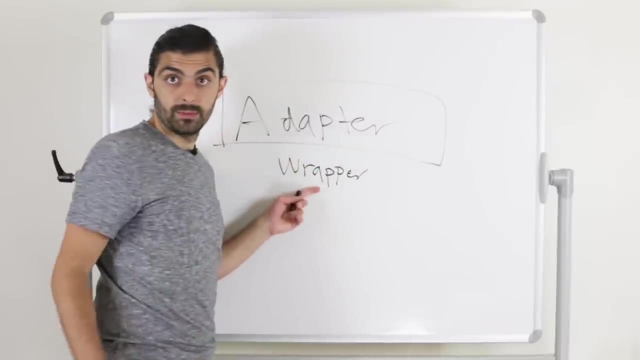 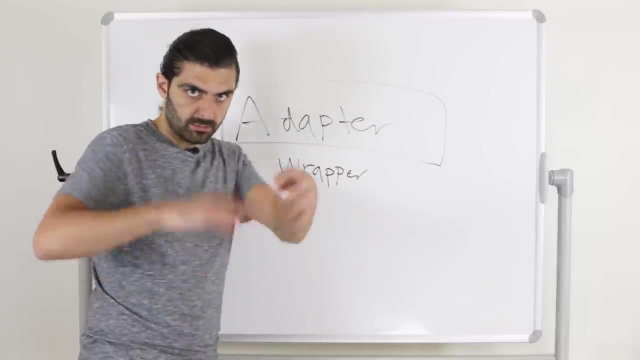 adapter pattern. Now, we're only talking about adapter pattern. By the way, the adapter pattern is also known as a Wrapper, a simple wrap, and this will start to make a lot of sense, because the adapter, what it does, is that it wraps Something so that you can adapt to a different interface. but now we're getting ahead of ourselves. but let's now get into it. 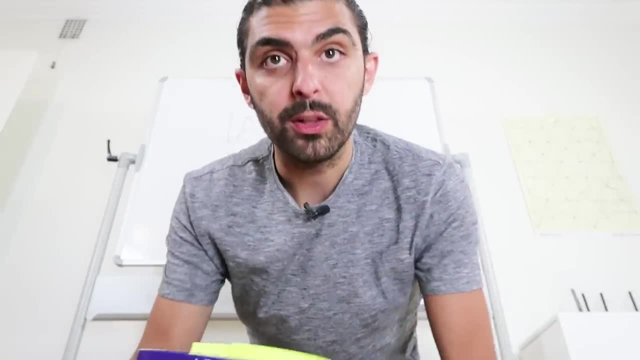 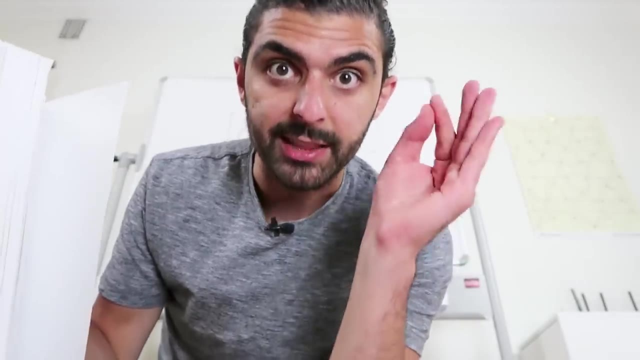 So, if you're new to this playlist or channel, What we're doing is that we're walking through all of the patterns in this book- headfirst design patterns- one by one, by one, by one, Which is now why we're at the adapter pattern and obviously, as you can see by what we talked about before, we will now diverge. 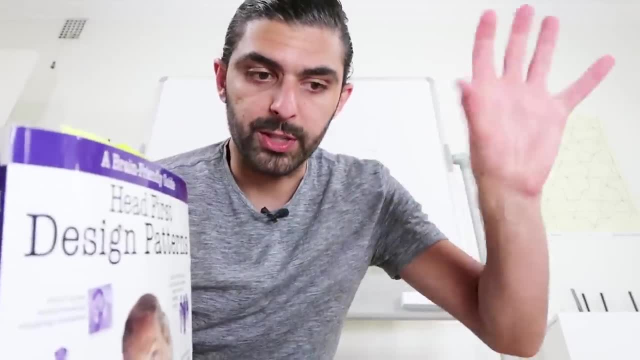 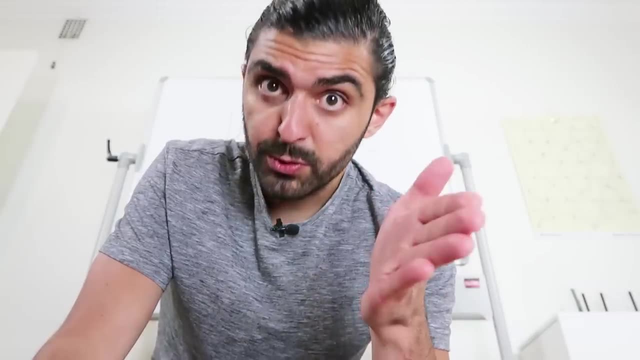 Slightly from the order in this book in order to be able to do that whole thing where we talk about the differences between these Patterns. so we'll put proxy pattern in a place for earlier than is in this book. But whatever. now, if you are new to design patterns, I would highly recommend that you get this book. It's super pedagogical. 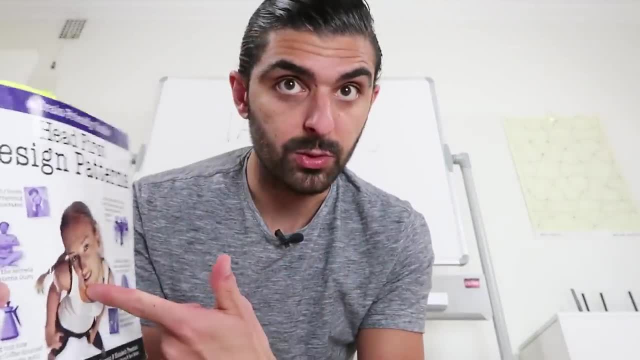 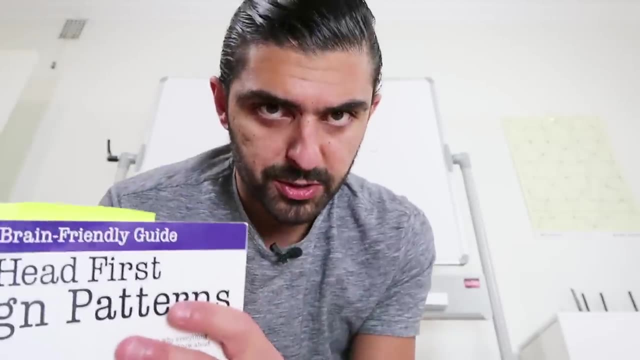 It seems super long, but the reason it's super long is because it has all these images and silly examples and like Fireside chance between different patterns and like tons of silliness. but Actually it might look stupid on the surface but when we actually start to read it 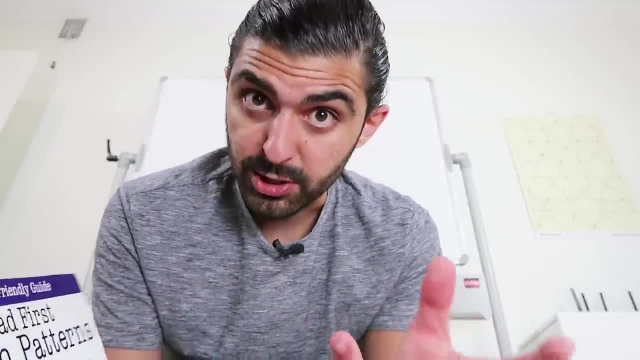 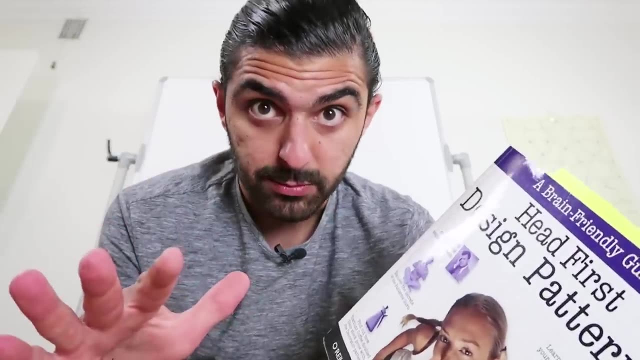 It's. they're actually diving into very deep concepts. They're actually trying to sort of trick us into learning very complex topics in a very easy way. So not at all bad. if you're new to design patterns. highly recommend it. if you're not new to design patterns. 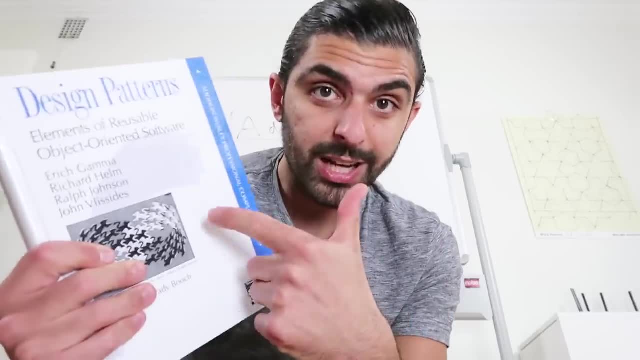 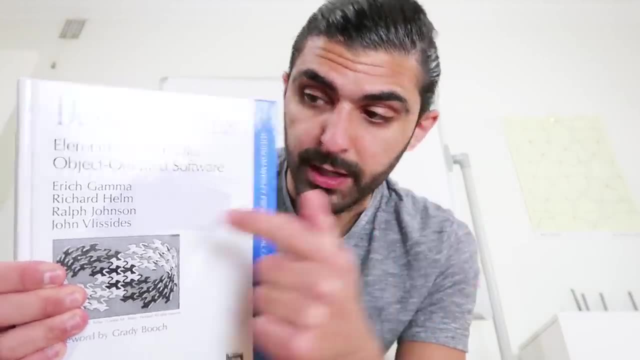 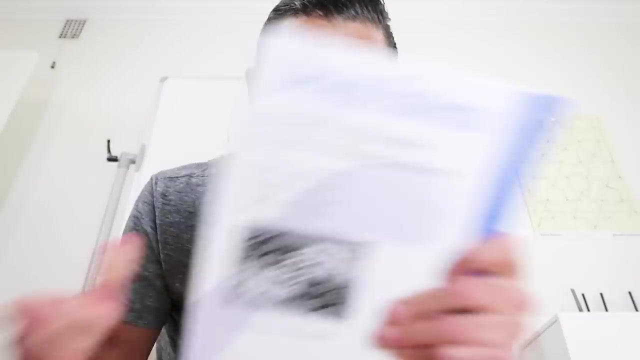 You know that I would rather recommend this book. This is sort of the classic gang of four book. perfect to put on your shelf: design patterns, elements of reusable object-oriented software by gang of four. This is much more like a reference book. So if you're new, I would again rather recommend this book because it's it might be disheartening if this starts to get confusing also. 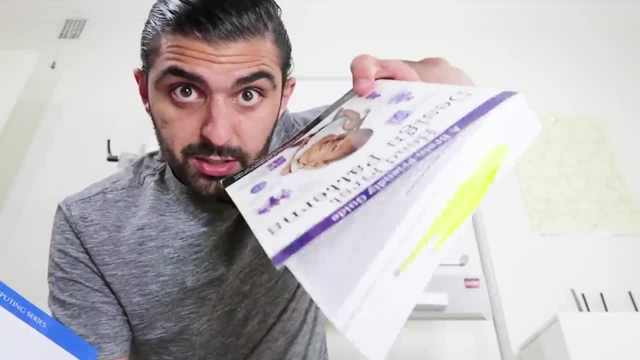 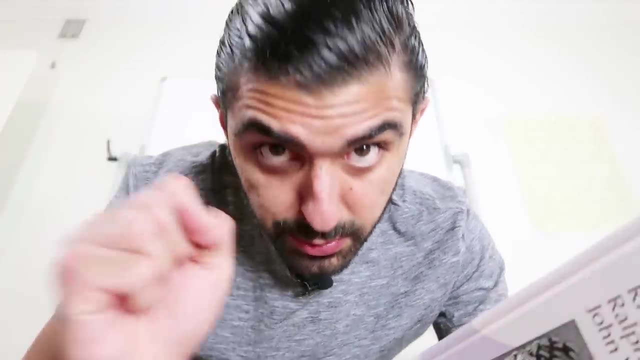 I think the examples are in C++, the examples here are in Java and of course, they get the best of both worlds. Yeah, the two of them links are in the description. with that other way, Let's move on into The adapter pattern. so let's begin by thinking about these now. What are these? 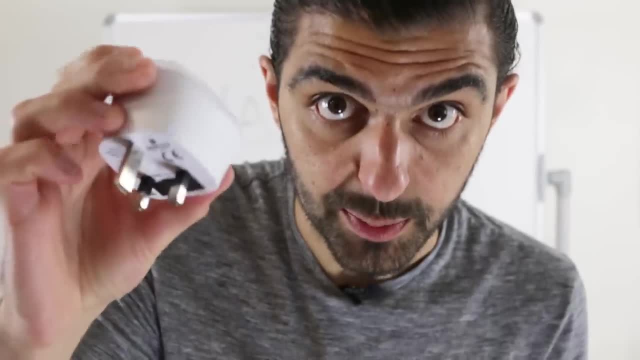 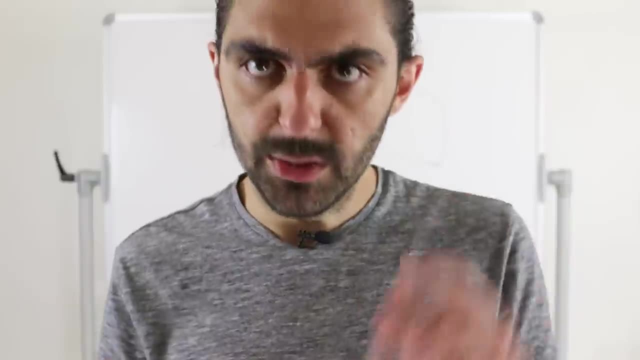 So let's just look at sort of this, most simple example. This is an adapter. if you're traveling, you might be from a country They uses one particular outlet- power outlet, one outlet, Maybe, it's a word, whatever- and you're traveling to a country where they're using different outlets. 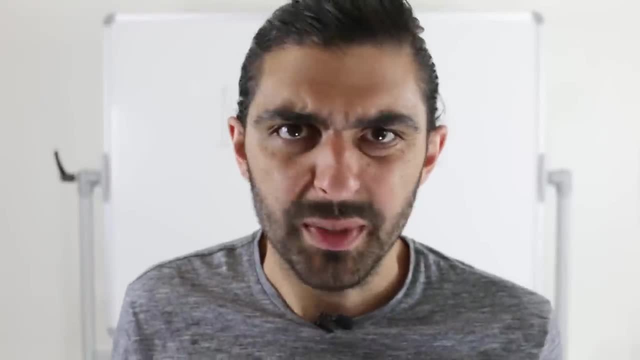 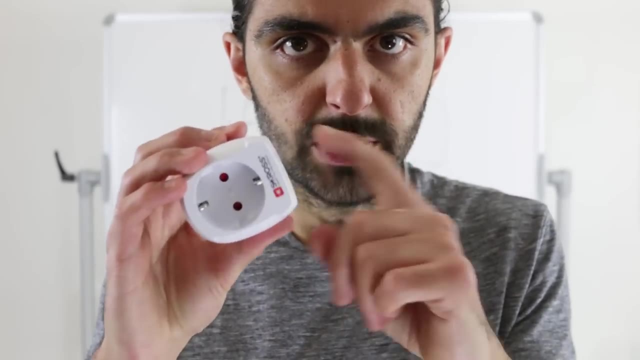 So this is the kind of socket that we use in Sweden- I guess it's like most of Europe except for UK- and it transforms this connection to a UK connection. So I'm from Sweden. I need this output. I travel to the UK. UK uses this kind of outlet actually. 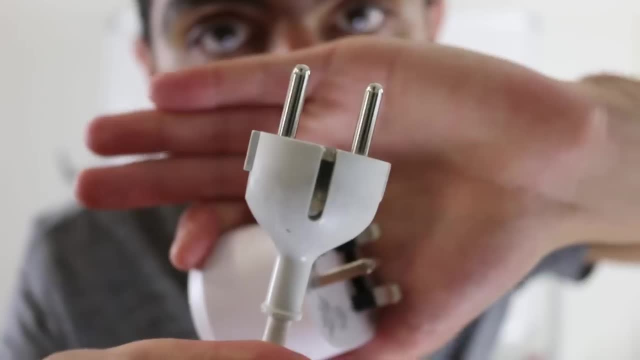 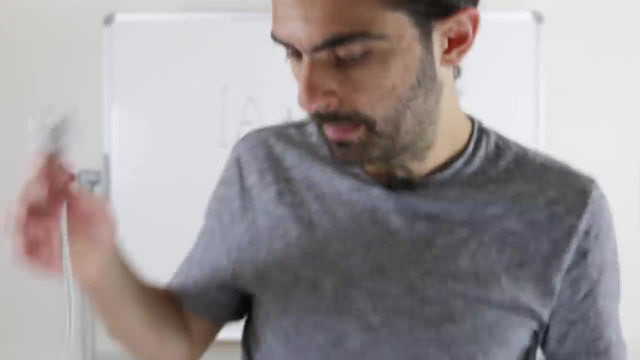 Let's get that. so I plug my MacBook charger- that looks like this- Into this and then I plug that thing into the wall. but you, You're all familiar with this. I mean nothing strange. and this is sort of the simplest type of adapter, right like you have. 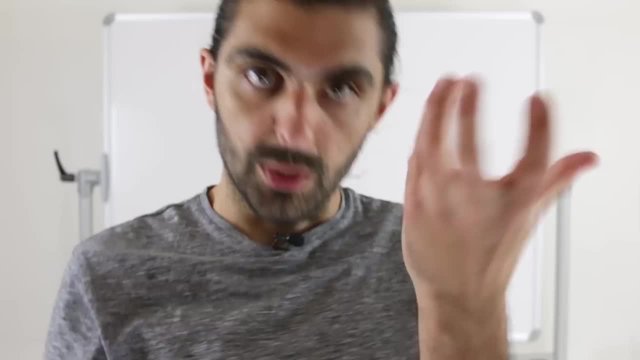 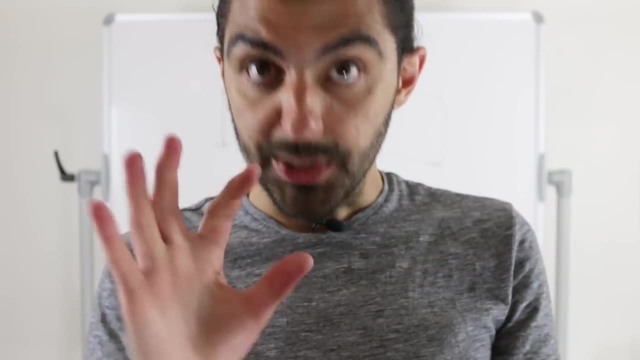 One type of input and you have one type of outputs. So you have something that's of euro standard and you need to connect it to something that's UK standard, and let's now start to use The, the word interface instead. So again, we don't mean interface as in Java or C, sharp interface. 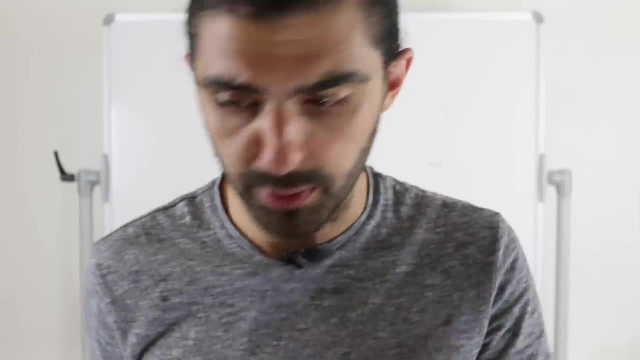 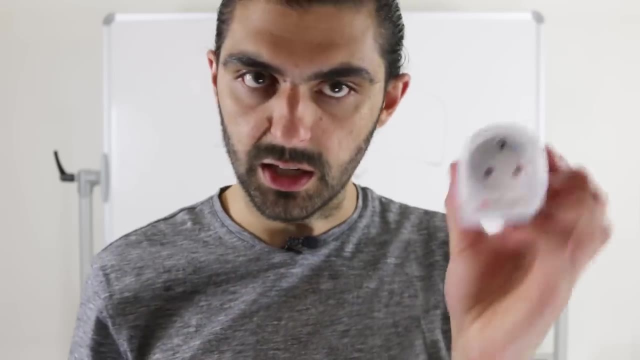 We mean interface in a way that, for example, this book and lots of other books use it. We use it to mean the contract between two things, right? So so an interface is like: this is an interface, This is the contract. like in the country, The contract is that if you have something that follows this particular interface, 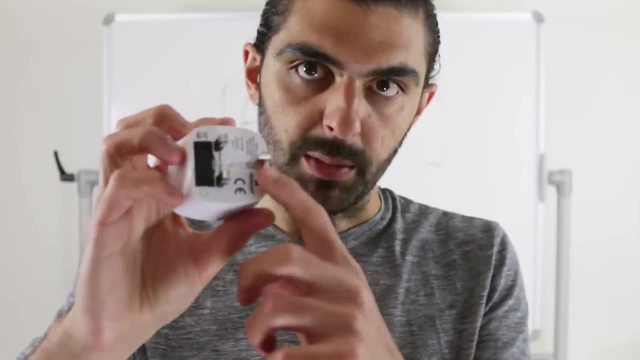 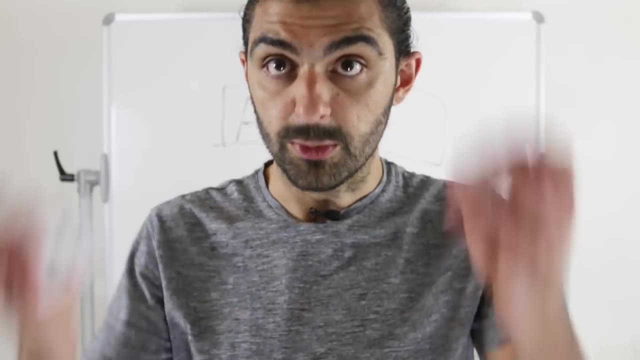 You will be able to plug it into the wall and get power. same goes in UK, But for this standard. so it maps us from this interface to this interface, from this standard to this standard. now, Of course, there are more complicated adapters like these, where this is, I guess us out and then as input. 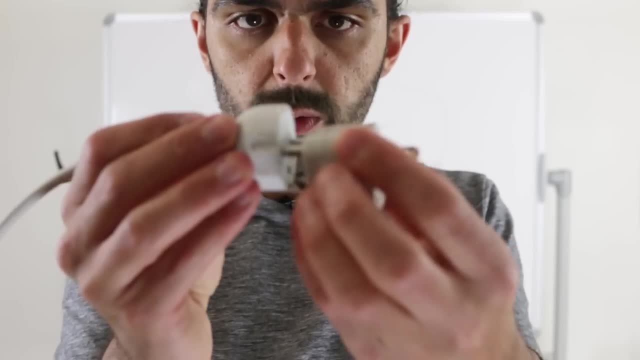 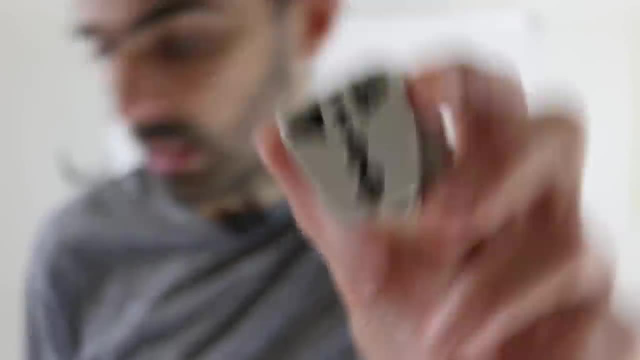 You can have lots of different things. So I believe my Swedish charger still works Well, good, but I mean I'm not using all of the holes here, So I would believe that a lot of other countries are still using it right. So the other thing that I would also like to mention is that maybe the adapter is supported by this particular adapter as well. 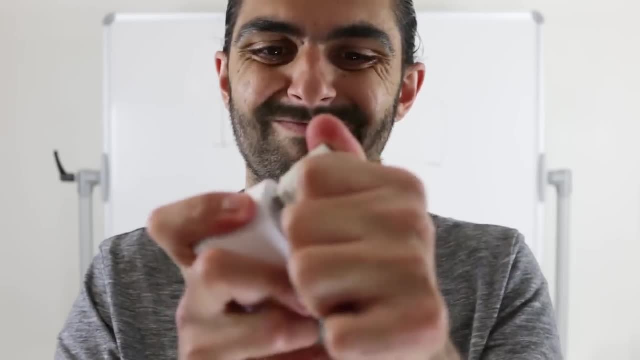 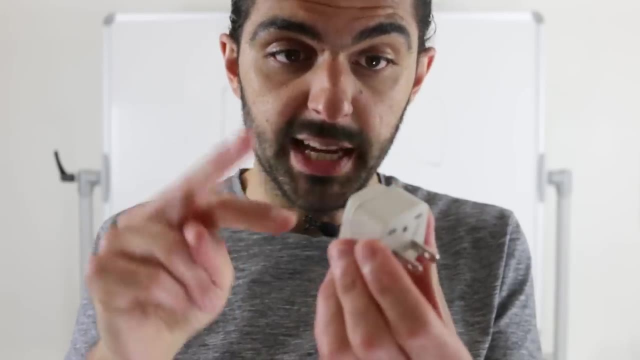 Maybe even- yes, maybe even- this UK adapter. So that works just fine, Doesn't? yeah, I'm not gonna break it. Who cares, It could potentially have worked. point is, this particular adapter takes multiple kinds of input and produces a single type of output, in other words, 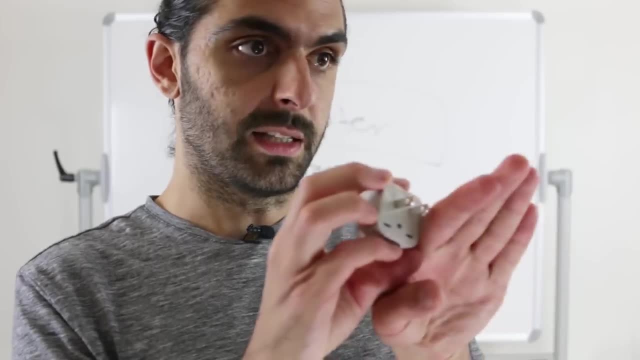 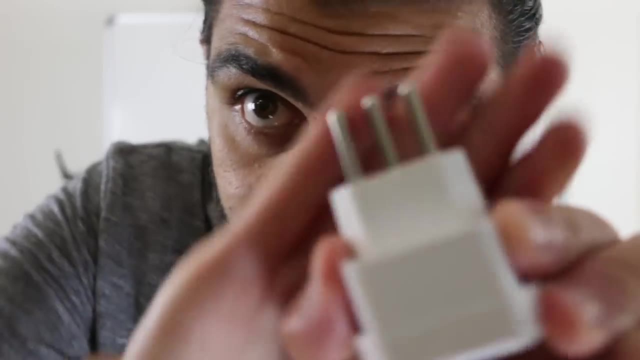 It's compatible with a bunch of different types of input and it converts that into one particular type of output. same goes for this one. that gets us to another standard. But again here we have one type of output, multiple types of input. These sort of more complex adapters we're not going to. 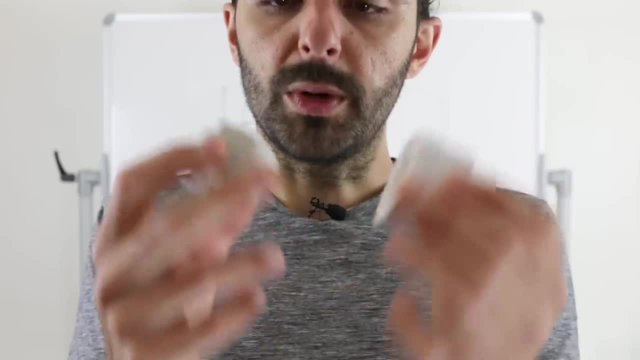 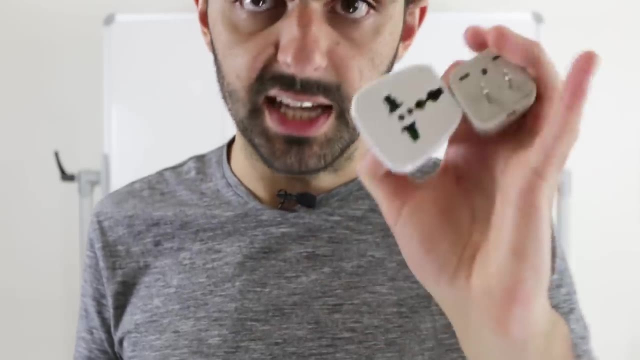 talk about explicitly in terms of code and metaphorically, but we're rather going to talk about this simpler one-to-one adapter. But probably you can see how it wouldn't be insane to construct these type of adapters. So you have one thing that has some interface, another thing that has another. 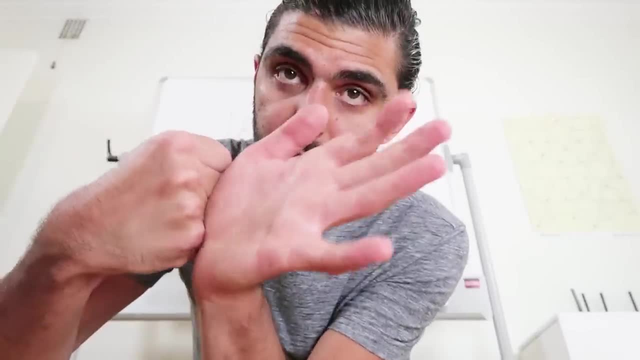 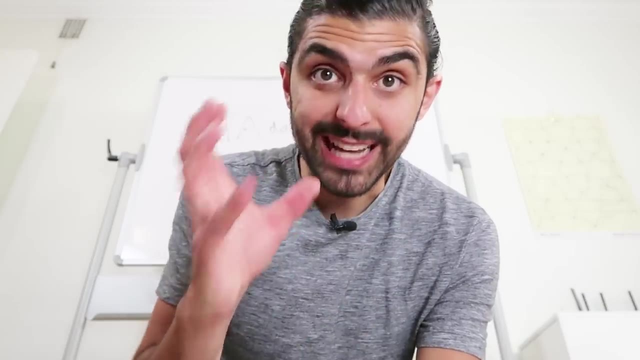 interface and then you create an adapter that you stick onto here so that the two things are compatible. Let's now look at the definition. So the definition from this book, head first, says: the adapter pattern converts the interface of a class into another interface. the clients expect. 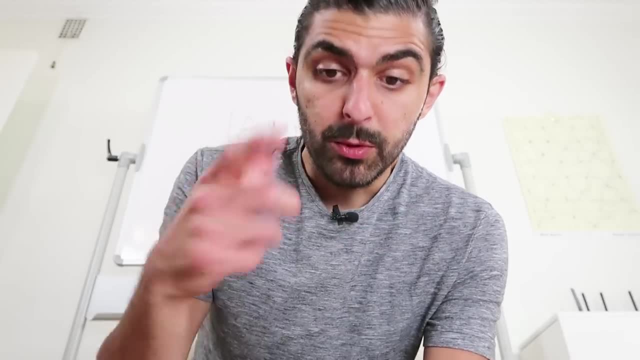 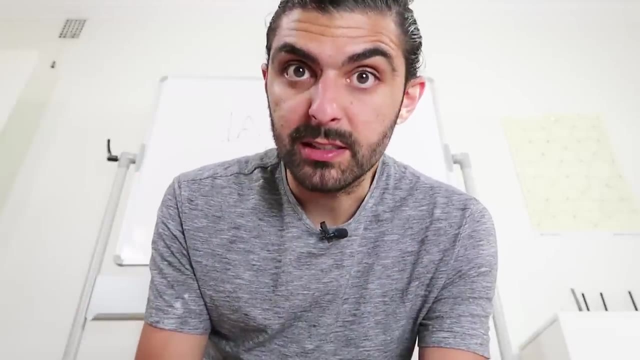 Remember, here again we're saying interface in the sense of the contract Moving on Adapter: lets classes work together. that couldn't otherwise because of incompatible interfaces. It's not that complicated, right. It's kind of what we were saying before. The adapter pattern converts the interface. 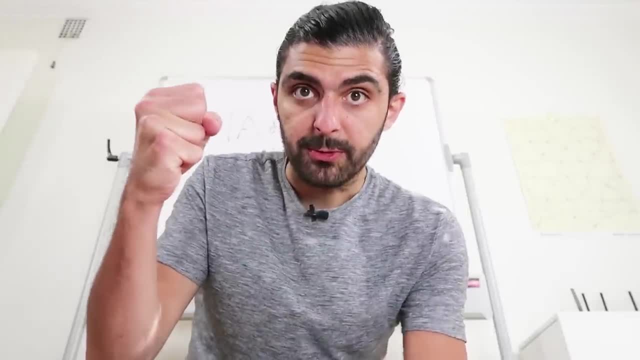 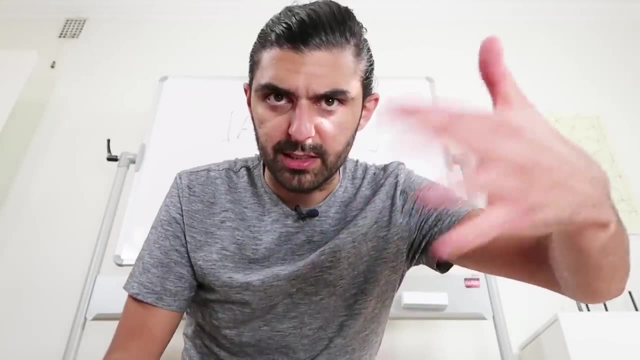 of one class, the thing we had here, into another interface, which was this thing that we were drawing here that the clients expect. so you have some client that expects this. we don't mean client as in customer, we mean client as in some user of the code, some other piece of the code that wants to. 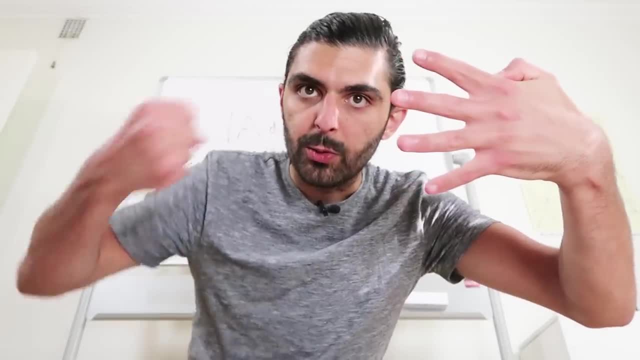 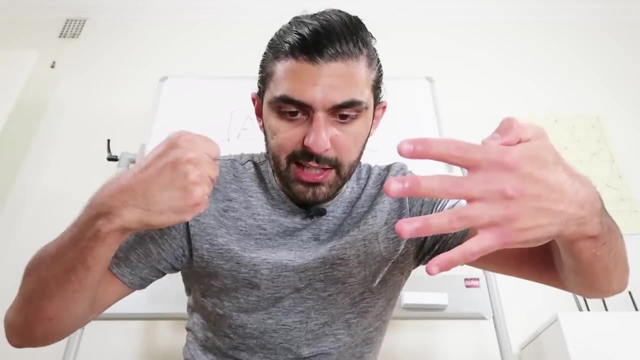 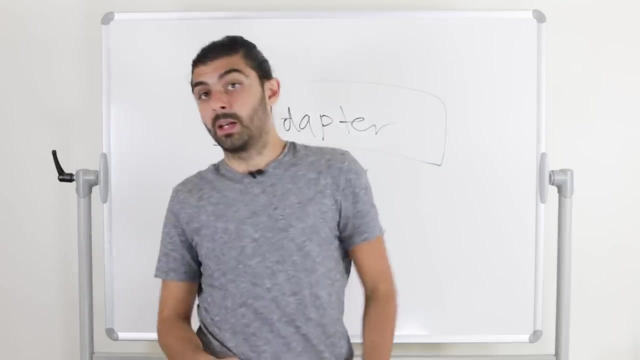 use the code. so this client expects this particular interface. but you have this particular interface and the adapter lets these two classes work together, even though obviously they can't now. so you attach an adapter to this particular object and suddenly you now have compatible interfaces. let's now look at uml. so let's remove this stuff and let's start with a client. so again, 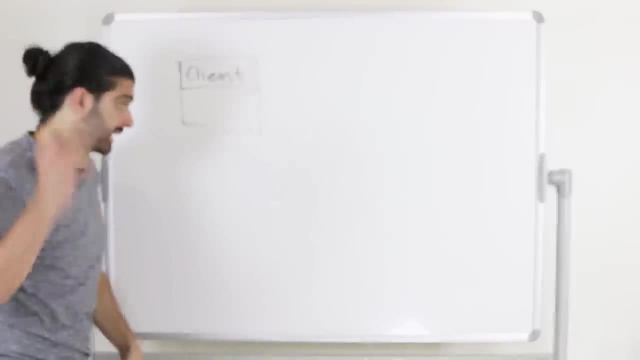 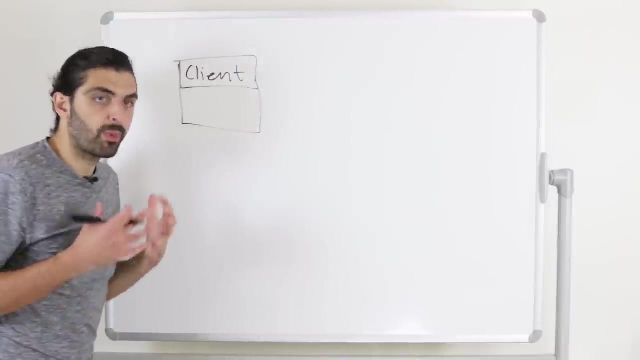 as we were saying before, this client refers not to a customer or anything like that. it refers to some piece of the code that wants to use something else. so this is the client here is not necessarily part of the pattern. the client is the user of the pattern in some sense. let's move on the client. 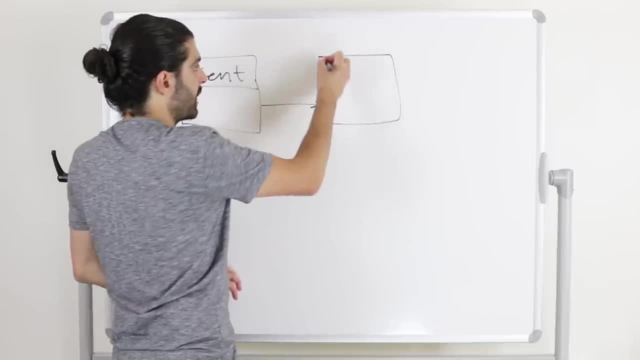 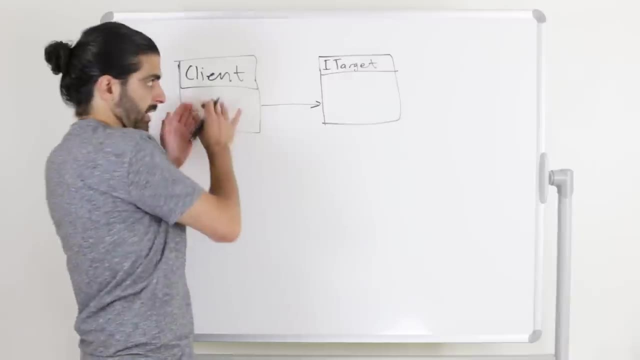 uses something which is of type target, but i'll put i target here to denote that it's an interface. this is not a concretion. this is an interface, so the client can't directly use an i target. it needs to use something that implements the interface i target. 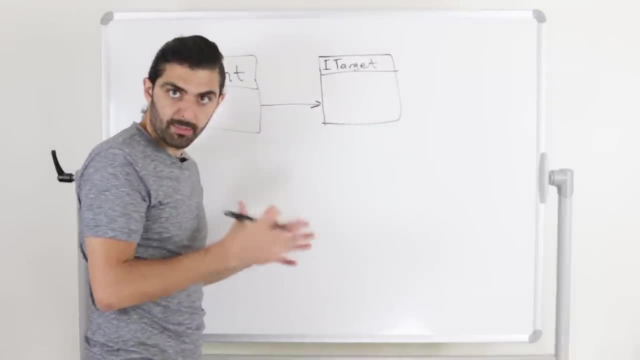 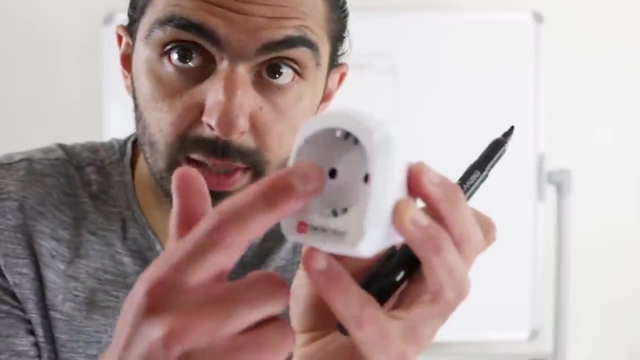 the interface i target defines that it needs to have a method, and this is the method that we want to call. this is the method that the client expects. this is when i have this. we are now in this end and not in this end. the client is used to using something like this: my macbook charger, right, i. 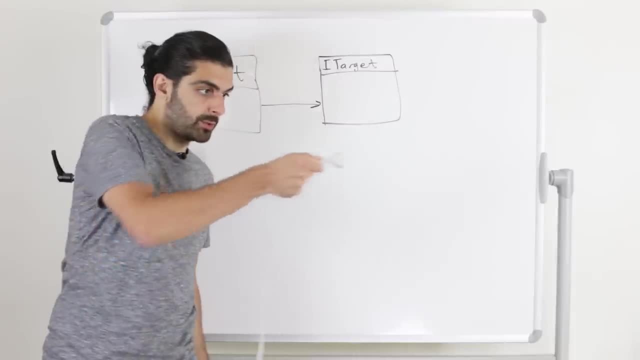 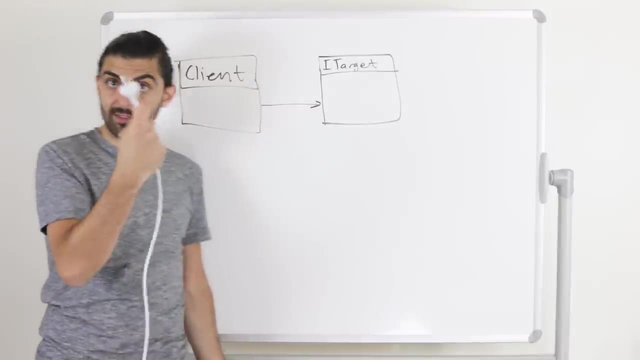 want to plug this in, but i can't plug it directly into the to the uk socket. i need the adapter in front right. but i but still like from my perspective, this is what i've got. i am the client and i have this. i have a swedish style or? 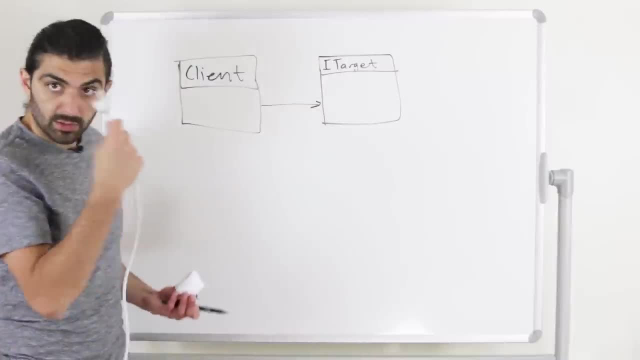 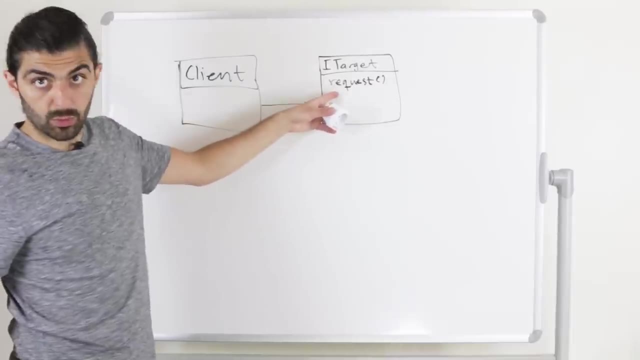 european style connector or whatever it's called, and i'm still going to use this right. so when we say request here, request, let's say it takes no arguments. when we say that i want to call a method called request, we're talking about this kind of thing. we're saying this is the signature of the. 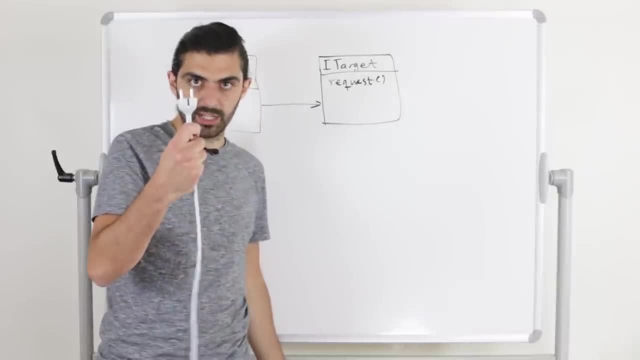 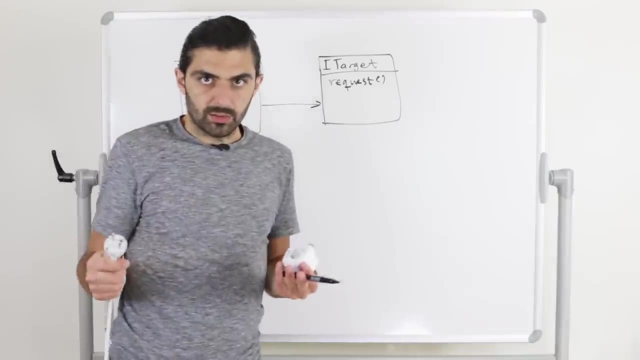 thing. i'm expecting, right, i'm expecting something to behave in this particular way. i'm expecting something to be called request. take no arguments and be a void method. of course, this could be, depending on your scenario, to be absolutely anything. it could be like you have a 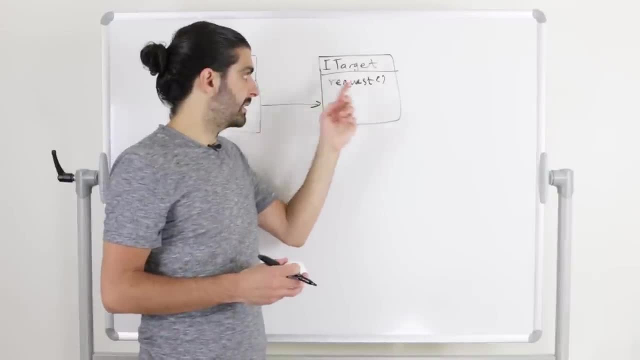 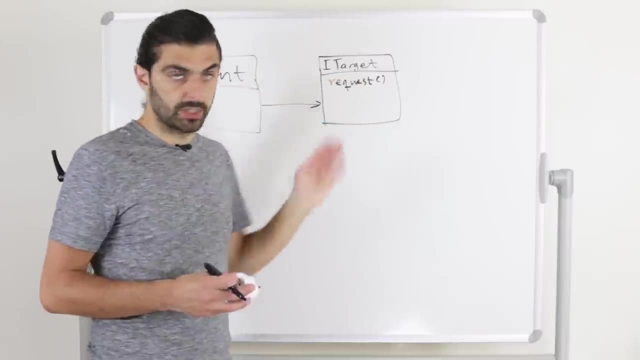 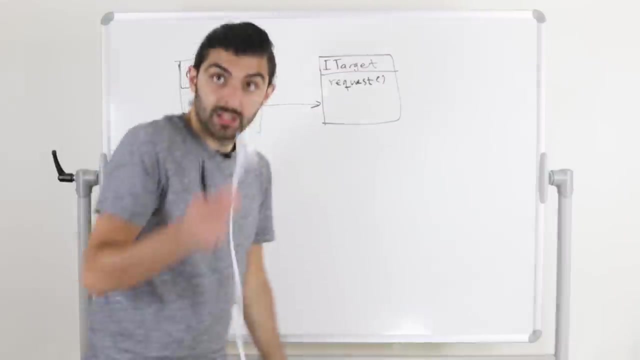 method called parse input that returns a string and takes a string and maybe takes a regular expression or whatever. i mean it could be arbitrarily complex. you have a method that has a signature and the point here is that the client expects a particular signature right. it expects this end, it is expects to be able to keep behaving as it's always behaved. the 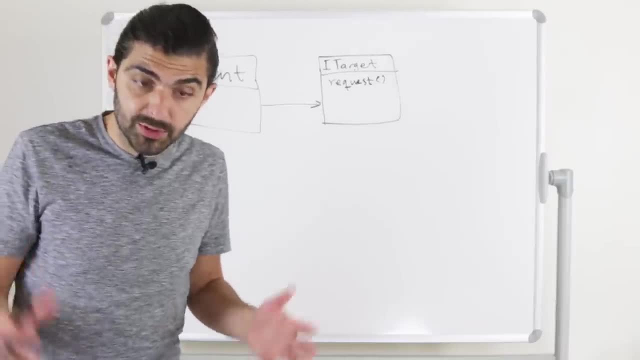 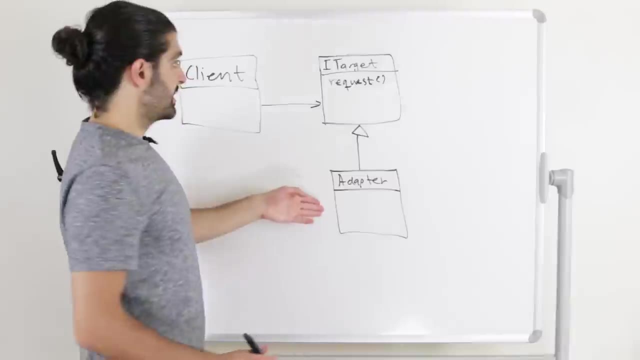 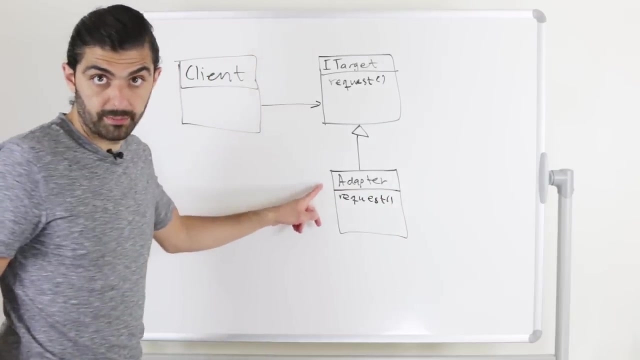 question is then: who implements itarget? that is, the adapter. so somebody called the adapter implements the interface itarget and since it implements the interface itarget, it needs to have an implementation, for the method request again takes no arguments and returns nothing. but the crux is that the method request is of this standard and this is why we're talking about. 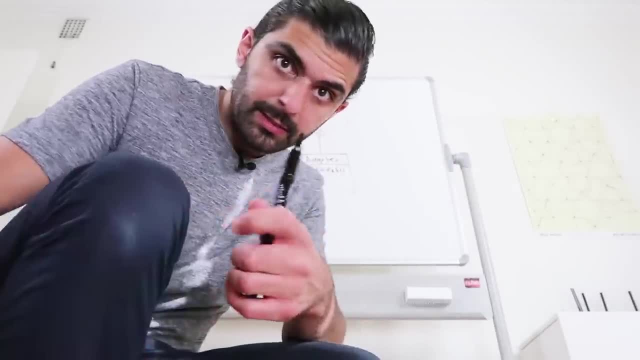 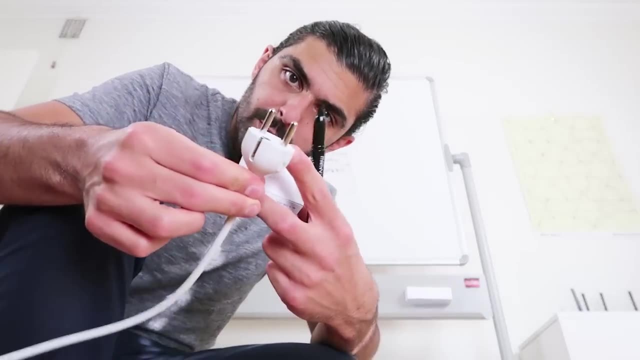 an adapter. we're expecting to be able to use this thing, this thing called request. but we are now in a place where requests need to be implemented and we're expecting to be able to use this thing. we need to look like this. so somehow we need to format, reformat, we need to reformat our request. 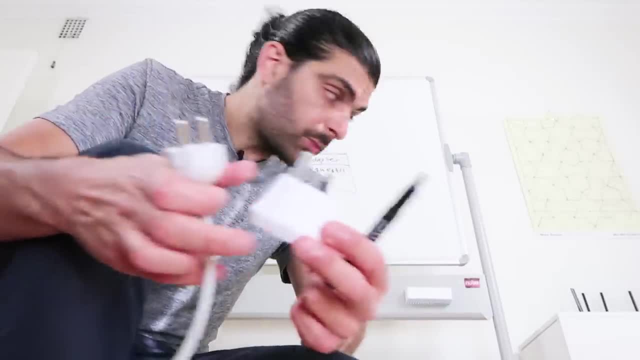 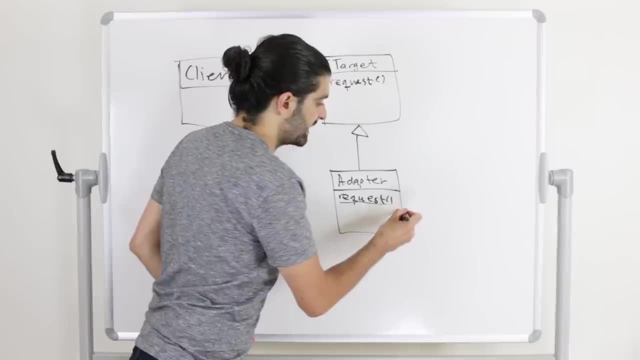 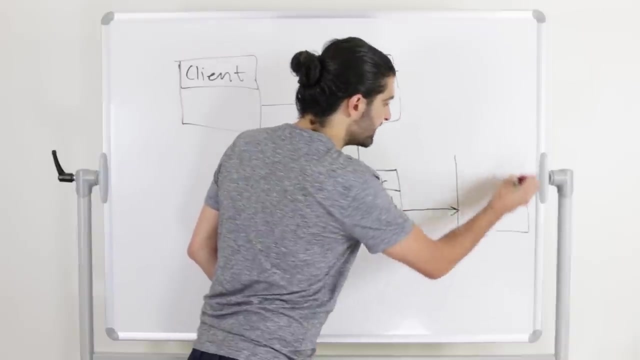 from this standard over to this standard. and how do we do that? well, that's the job of the adapter. so this adapter is taking in a request call, but it delegates to remember this error is hazard. it delegates to another class something which follows a completely different contract, a completely 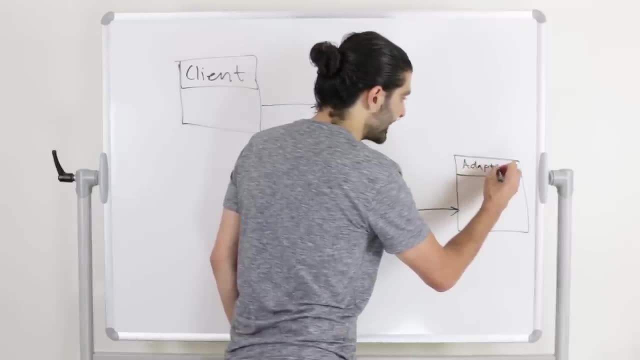 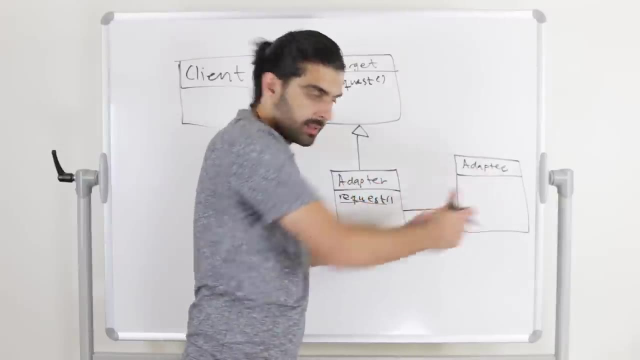 different interface and we'll call that the adapt t. we're calling it the adapt t because it's the adapted thing. so an adapter adapts an adapt t. i'm not sure if that's actually a real word, but that's what they're using in all the books. so whatever, actually it makes a little sense and 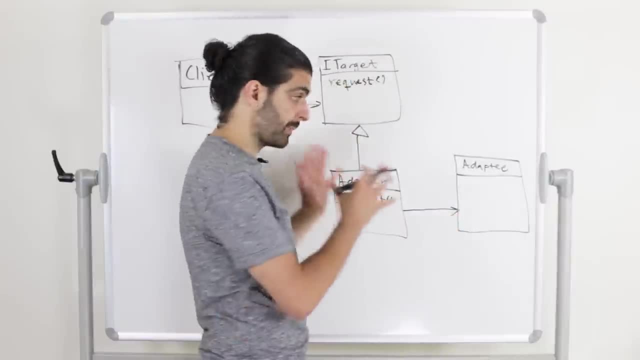 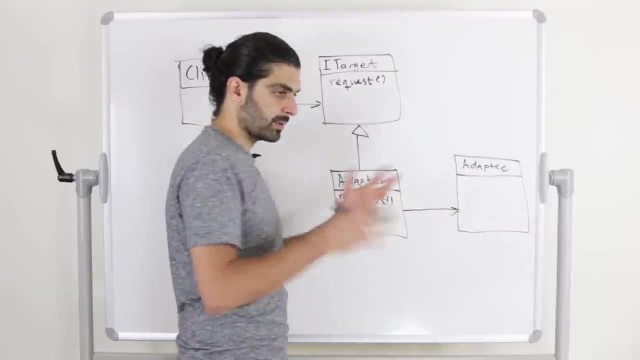 here. of course, again, these method names are completely arbitrary and depends on your scenario, but in order to show that this method completely could be anything and is not necessarily the same as this method or, i should say, doesn't necessarily follow the same signature as this, this method. 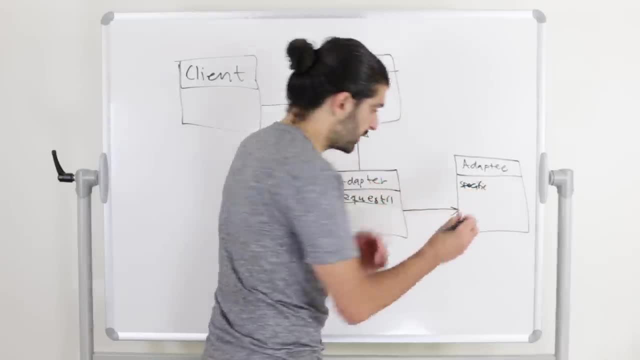 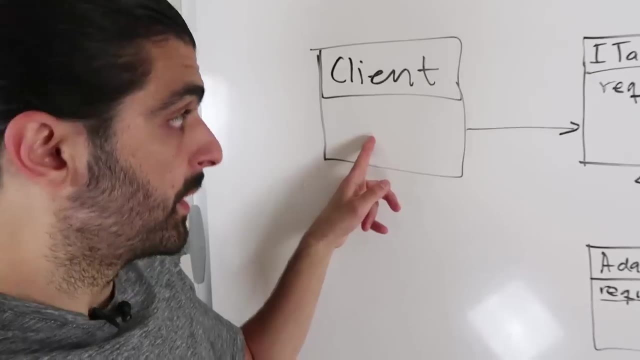 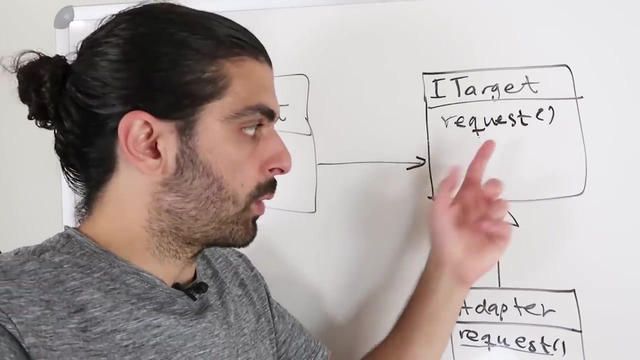 we'll call it specific. so sorry about the small font. request: specific request. so let's follow this along. the client, the user of the code, has something of type i target. this i target has a method called request, and request is the standard that we're used to using. but because 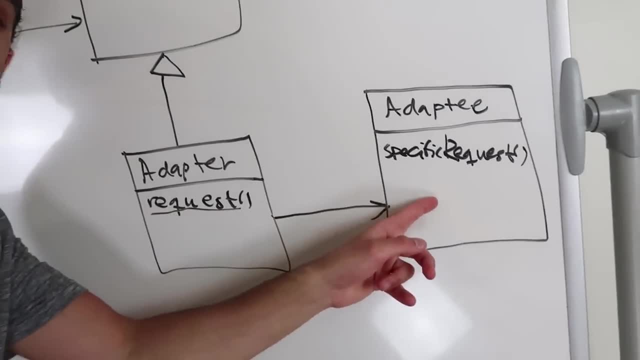 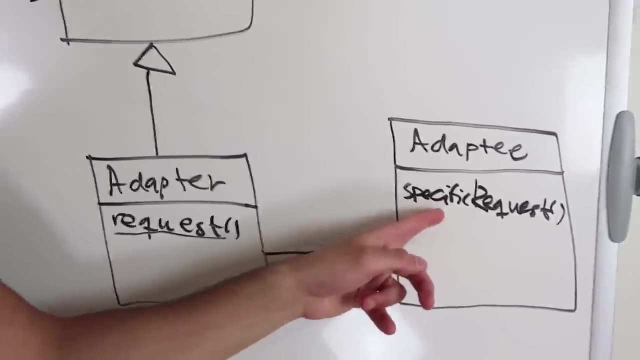 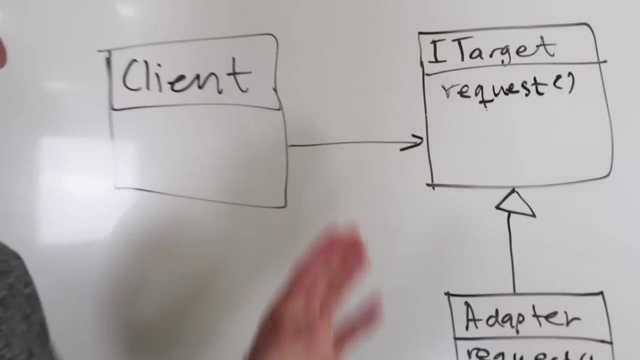 we want to use something that has a completely different interface, the adapt t. we can't just call request, because adapt t does not have a method called request. adapt t has a method called the request method, but we invoke it on an adapter, so the adapter follows the signature that we're. 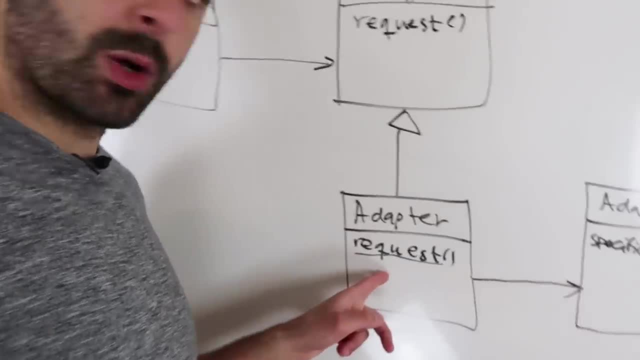 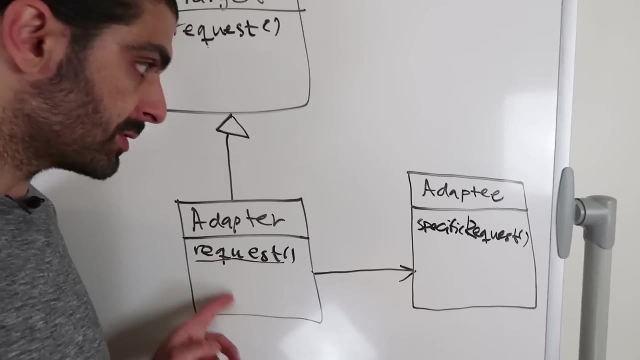 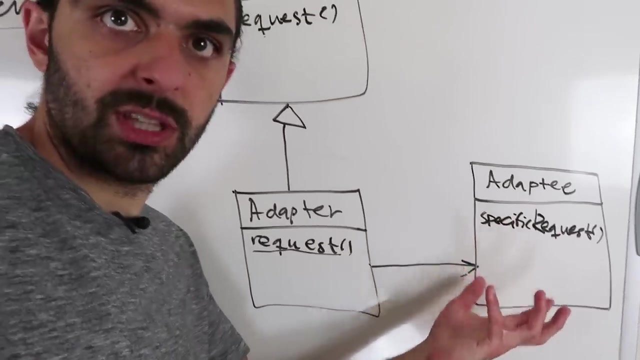 used to using it follows the signature request, so we can call request and then count on the adapter to call the adapt t. because the adapter has an adapt t so it is responsible for delegating the request down to the adapt t and then the adapt t uh can perform that specific action that we 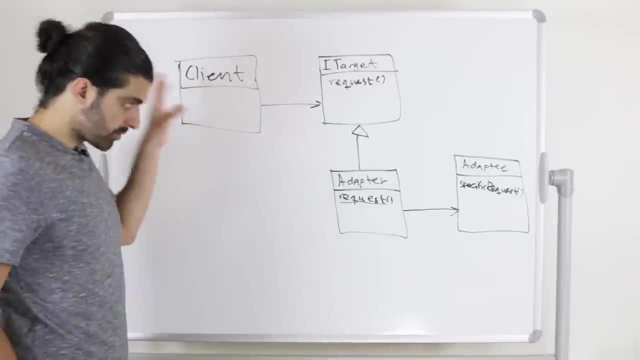 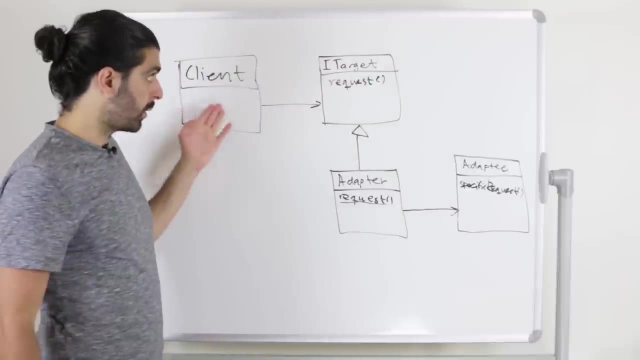 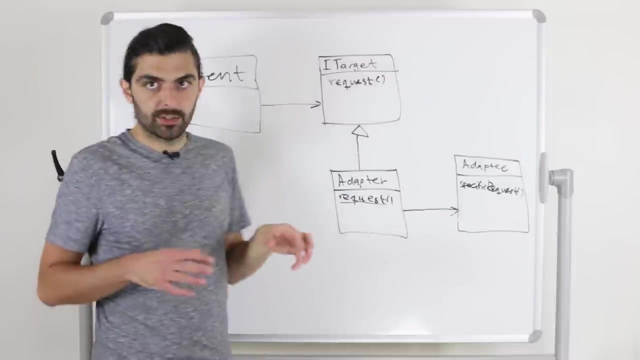 were originally interested in. so the client is, for some reason, wants to call the request, this method specific request, but for some other reason, it wants to call it using this particular signature, using the signature request to contextualize this. it could be, for example, that this particular standard is scattered across a lot of different places, so it would be painful. 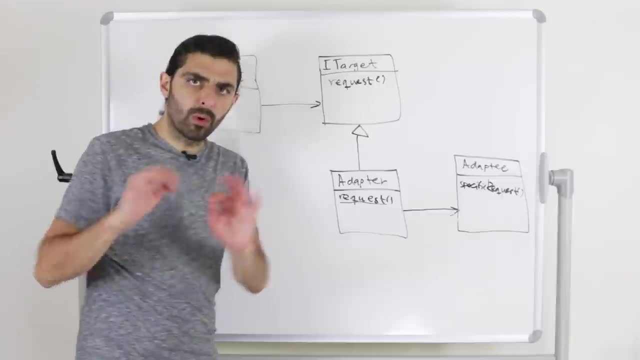 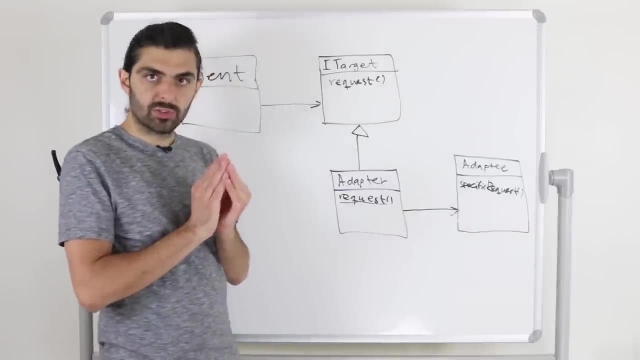 for us- we imagine- to change it to, to this particular style, or it could be that we envision that in the future we might actually want to change the signature. so we want to encapsulate that potential change in a place so that it will be easy for us to change in the future. 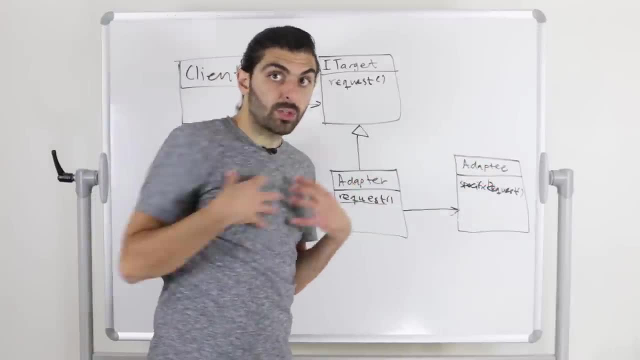 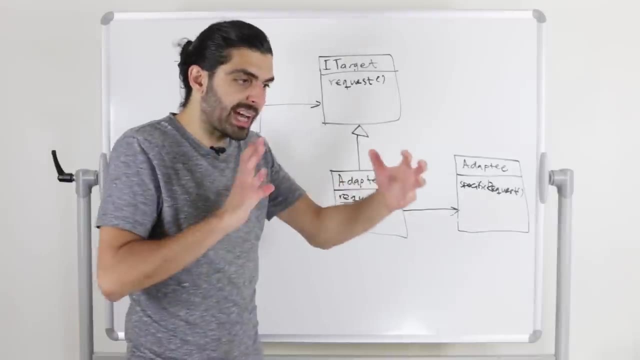 it could be that this adapt t, for example, is an external library that we don't actually have control over, and but we're not sure that we actually want to use that specific library forever and ever and ever. so we wrap an adapter or we put an adapter in between the two, so that 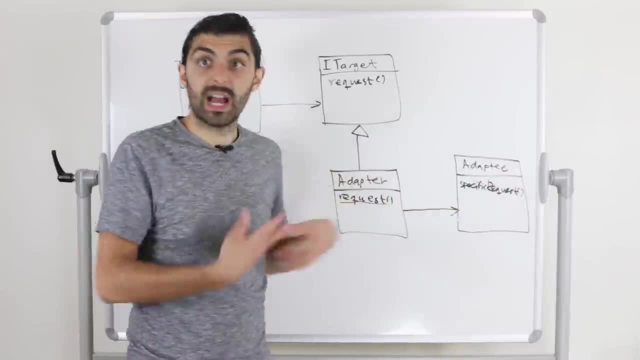 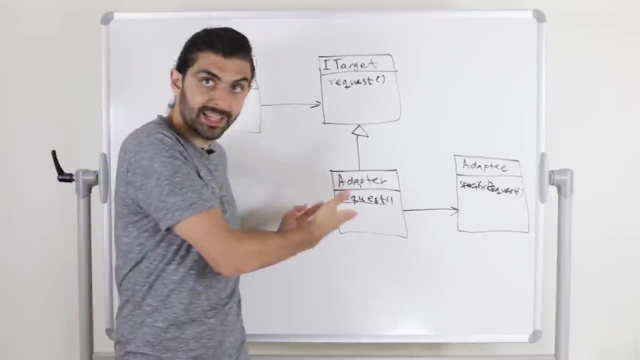 if we change our minds about what we want to adapt, what we want as our adapt t in the future. we can kind of trivially exchange that because we just switch out the adapter or make the change in the adapter but the client, in other words, want to call the method specific request, but it wants. 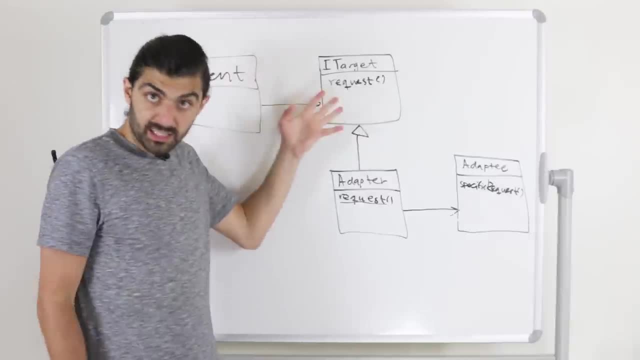 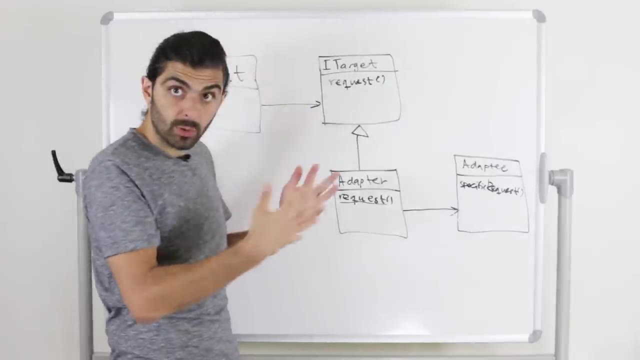 to do so by using the the signature request, and that's fine, because in order to be able to achieve that, in order for the client to be able to call the method using the signature request, even though the actual underlying signature is specific request, what we do is that we stick this adapter. 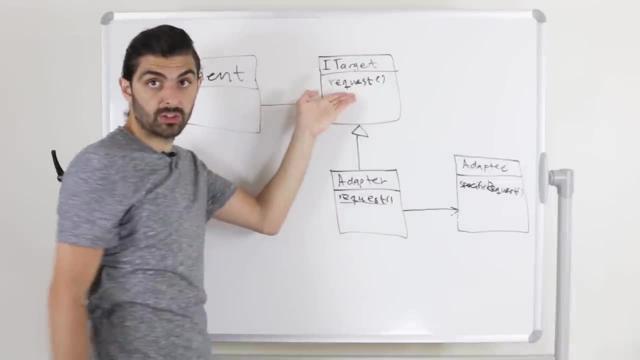 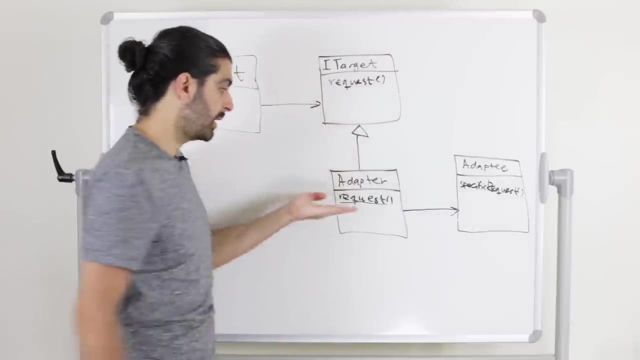 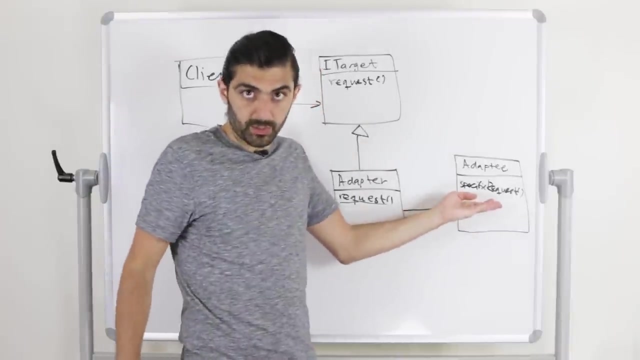 in between. so the client couples to an interface called itarget that follows this particular interface that it wants to follow, and then we have a concrete implementation of this particular interface, called the adapter, which follows this implementation. and when called, when we call the request, we then invoke this specific request, we then use this other signature. so we stick this. 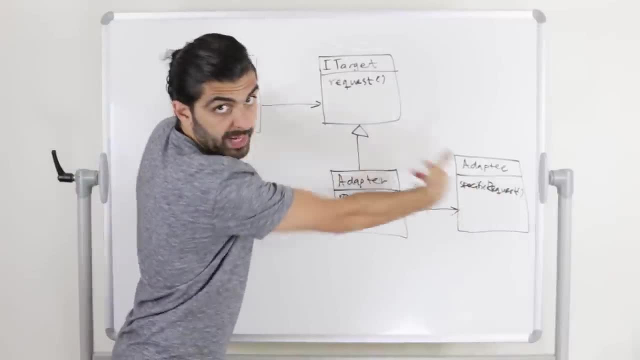 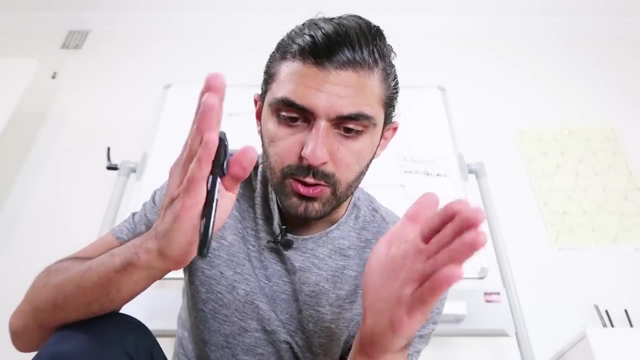 in between the two so that these two things are now compatible. and that's really it. that's the adapter pattern. let's quickly look at some code, but before we do that, let me just quickly mention that the intention is to not change the underlying behavior. you adapt something, you have an adapter. 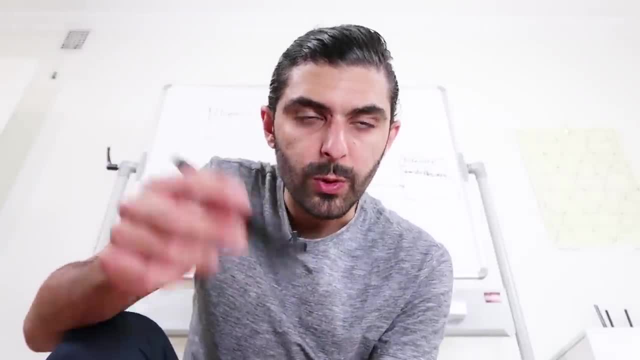 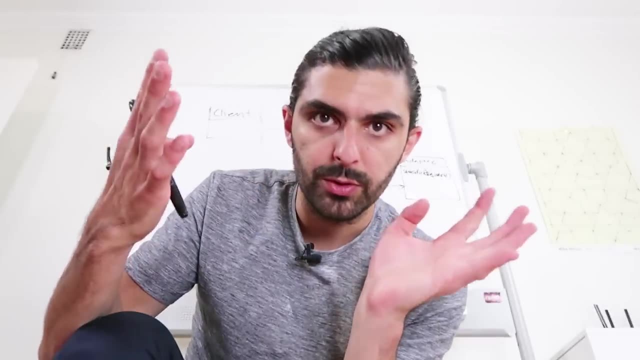 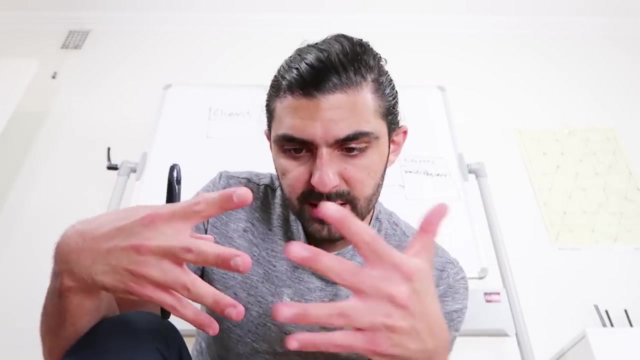 that you stick in between two things. but the intention is not to add behavior, it's not to remove behavior, it's not to alter behavior. the intention is really to somewhat blindly just pass on the request. the point is that you have two different types of signatures, you have two different types of interfaces and the interfaces don't connect. 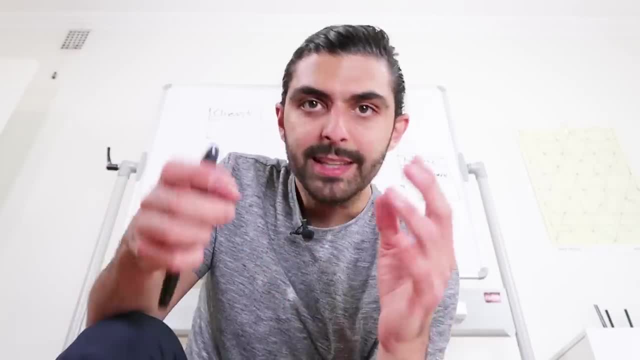 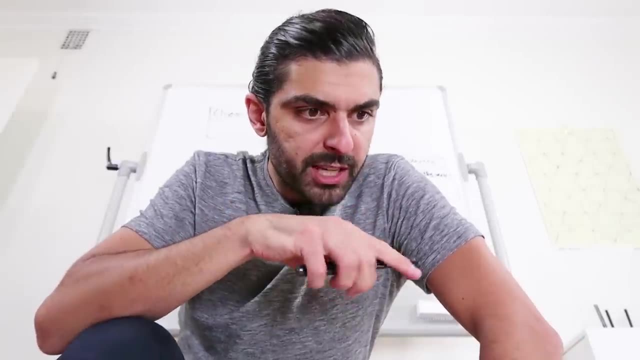 they aren't interoperable, so the intention is to make them interoperable. the intention is not to add additional behavior. think about it this way. i'm not an electrical guy, so please forgive me if i get this wrong, but different countries have different voltages right in the outlets, so what? 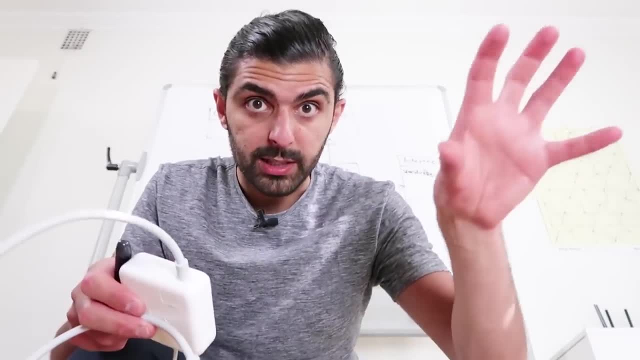 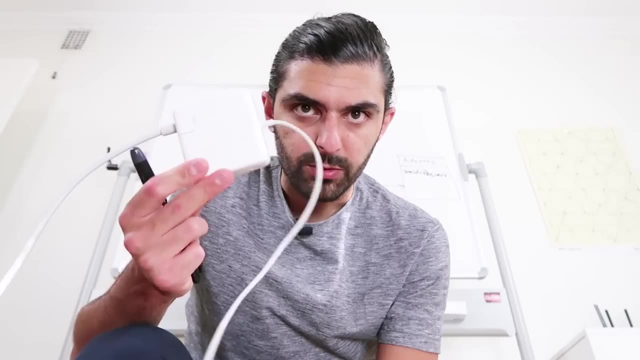 i'm saying is that in sweden we have one voltage in the outlets and the wall outlets and in the transformers we have a different voltage coming out from the outlet. now, probably in any modern device this is solved in the transformer- i guess this is called. but the point is that if we didn't, 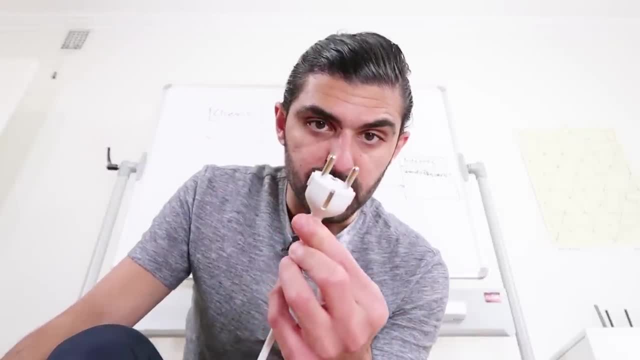 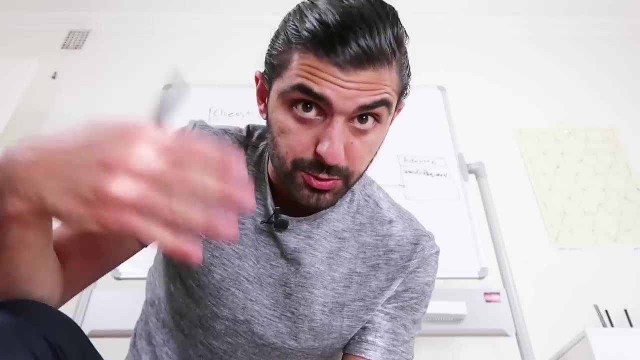 have this transformer. it would be potentially dangerous for for our devices to simply just put, stick an adapter onto our thing and then connect to the socket, unless we didn't have this transformer that also transformed the voltage to what was expected by our device. so if that were the case, 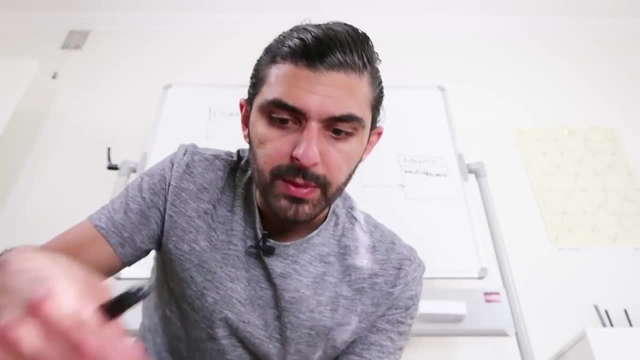 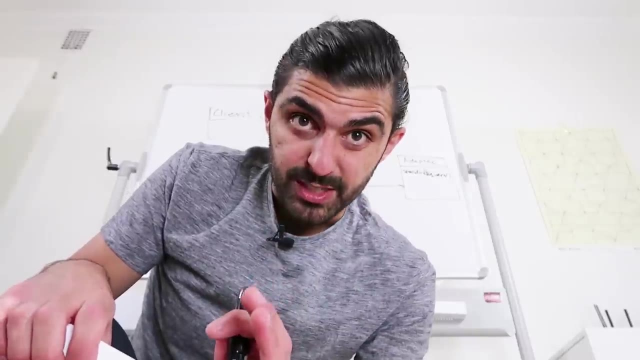 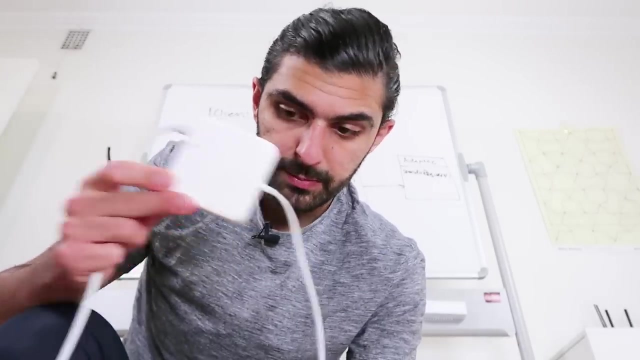 if we didn't have this transformer and we needed to, in other words, alter behavior. we're not talking about an adapter. we are talking about something else. potentially we're talking about a decorator, but we'll leave that for this specific video. so the adapter is not this thing super important, because this thing actually has intelligent logic. 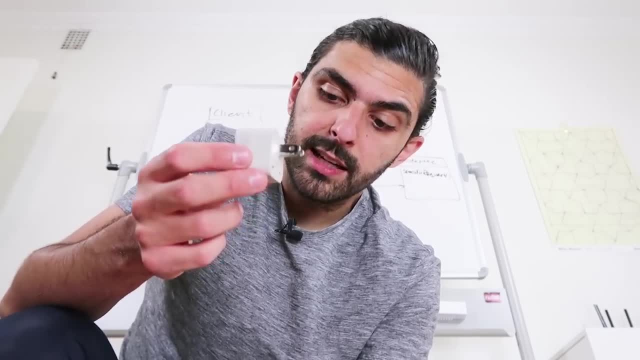 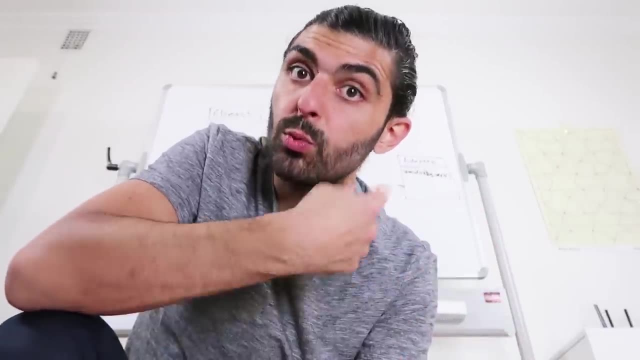 of course, this might be somewhat intelligent, but again, the idea is that the behavior of the thing that you're adapting, the adaptee, the behavior of the adaptee, is the actual behavior that you want. you want that behavior. it's just that you can't get to that behavior using the interface that you. 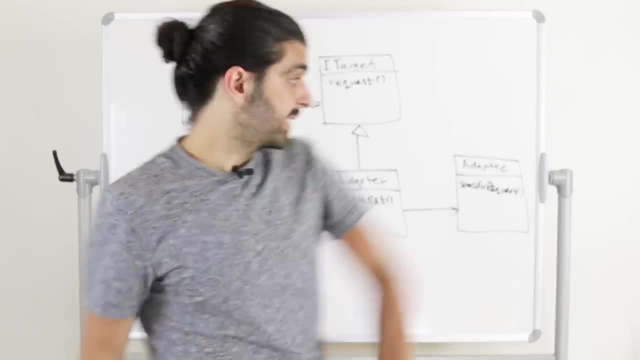 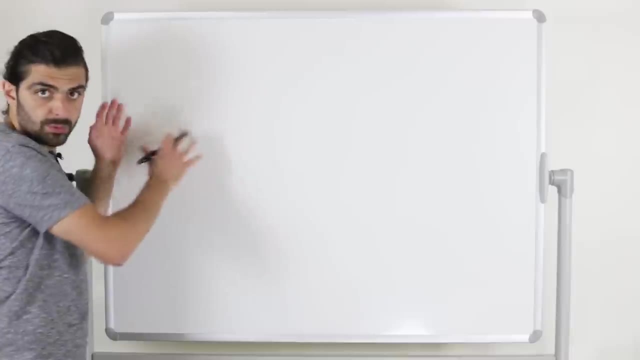 that's it. let's now look at some code. all right, let's begin by deleting this stuff. so let's start in the client end. in this end we have the client, so let's just say that we had a client i. i won't draw up the class, but just assume that i'm in a context where i can execute some code. so what we? 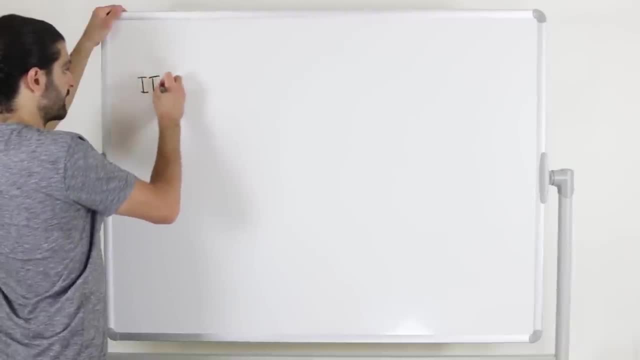 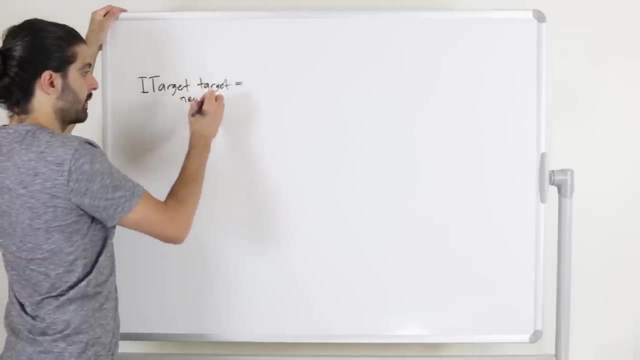 do here is that we would want to have an i target- let me put that in a variable. i'll call target lowercase- let me just break the line here to save space- equals a new adapter, and this new adapter has a constructor that's called a new adapter. and this new adapter has a constructor that's called a. 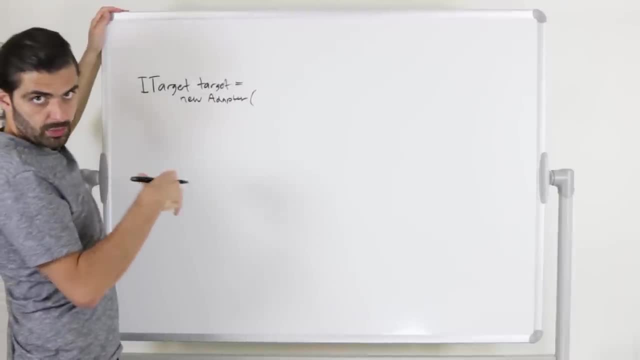 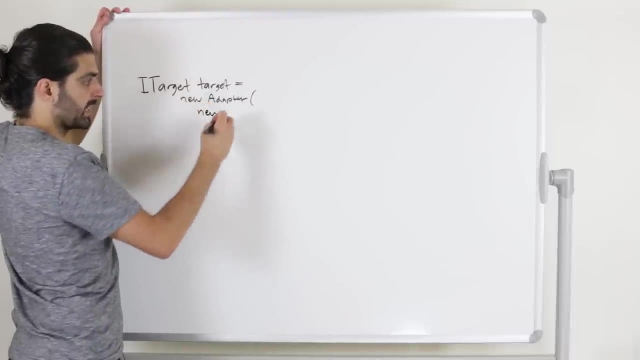 new component. that takes an argument which is the thing that it wants to adapt, the adaptee. and the adaptee we said had the type adaptee. so let's say new, again breaking the line adaptee, and of course you would pass whatever that takes as arguments. but now we don't know. 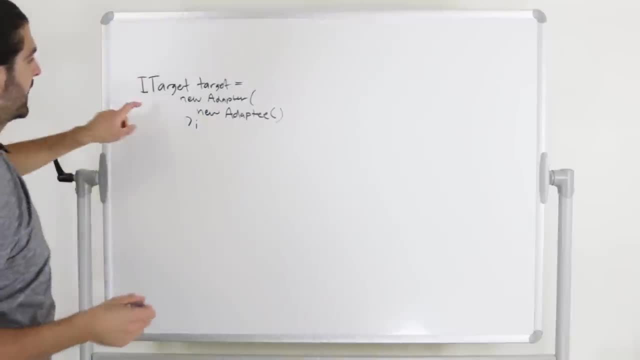 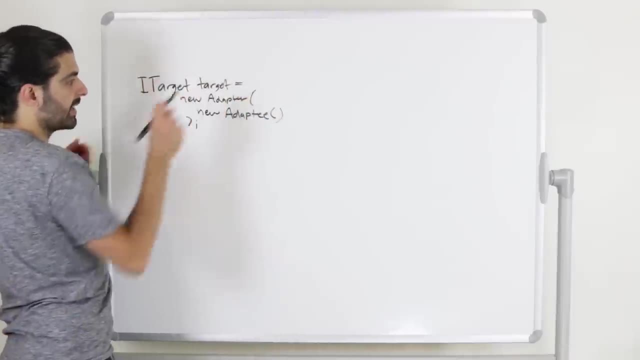 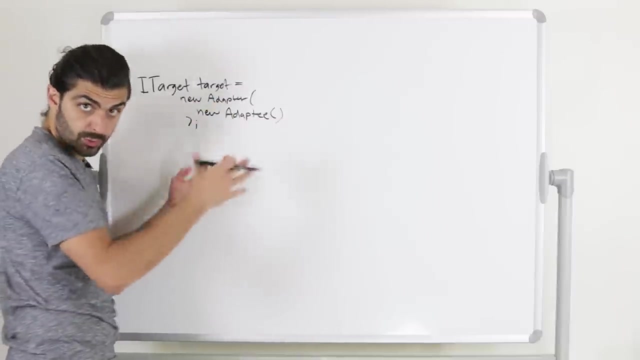 and i'll just close this parenthesis here- semicolon and we're done right. so there's a variable of type i, target the, the interface that we had here. the variable is called target and it contains a new adapter, the concrete adapter that we had roughly here, and to the newly created adapter, to the constructor of the adapter, we pass an adaptee. The reason we 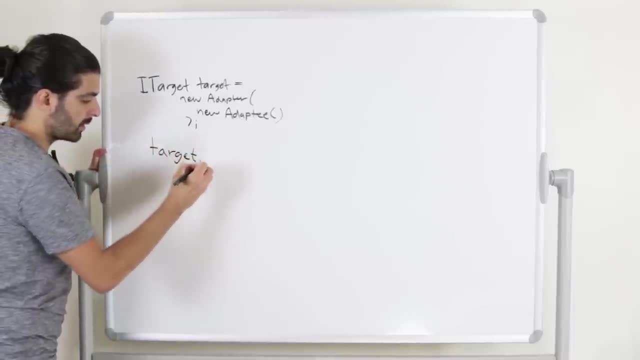 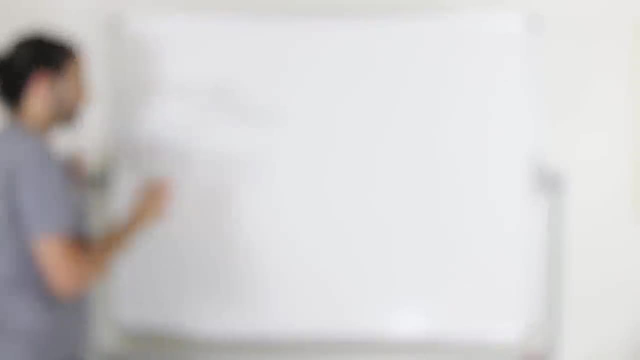 do this is that we want to be able to say targetrequest. This is the method that we actually want to invoke. That's the standard that we were used to. So, again, you have to imagine that this particular piece of the code could potentially happen elsewhere. Of course, this is the thing. 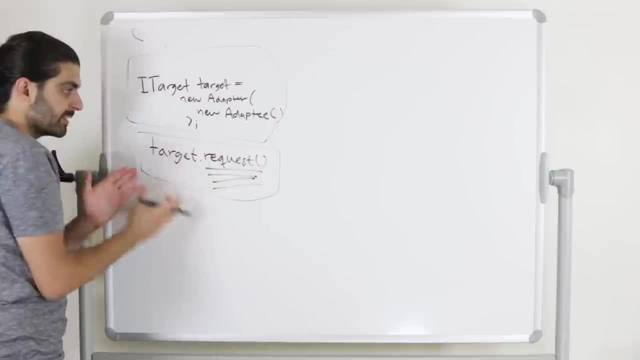 that we're interested in and we were in a context, we were in a client where this particular logic happens. So, again, this particular client might actually receive the target rather than instantiate it here, but that's a completely different story. The point is we want to invoke this method. request. 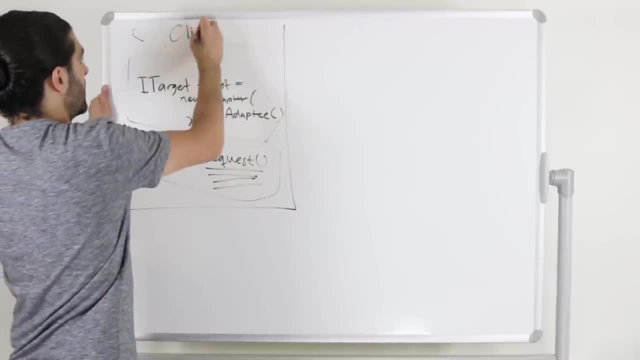 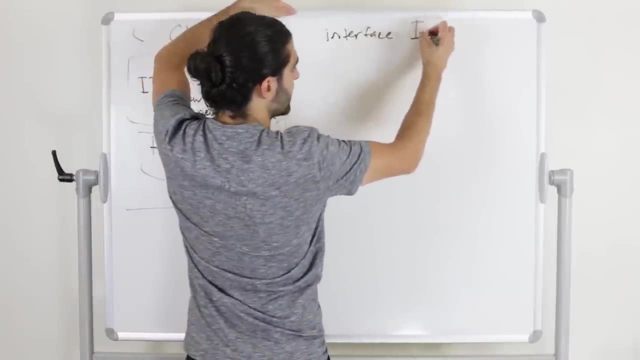 Now what do the other stuff look like? So this is the client Client. Then we have- let's start with the itarget. So the itarget is easy. It's an interface called itarget, Super easy. It just does one thing: It says to be something that implements the interface itarget. you need to. 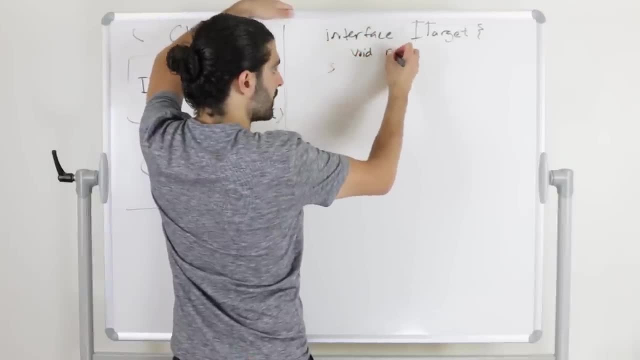 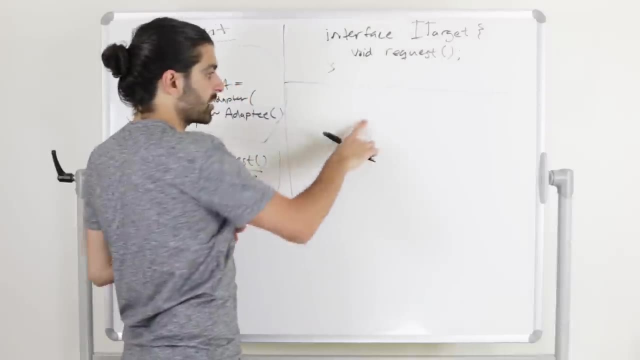 have a method that returns, void nothing and is called request And takes no arguments. That's it, Okay. Next thing, That's the interface. Then what was our actual adapter? Because the adapter is the thing that implemented the interface itarget. So let's. 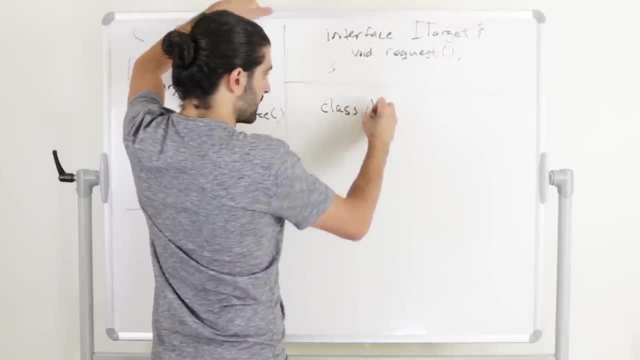 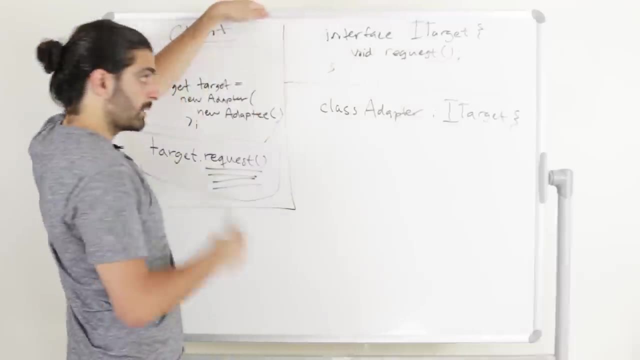 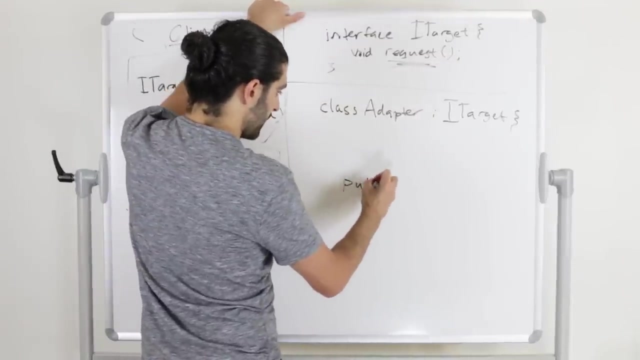 build the adapter. So the adapter is a concrete class Class called adapter, And it implements the interface itarget, And to do so it of course needs to have an implementation for the request method. So let's build that method. So the class adapter needs to have a method that is public. 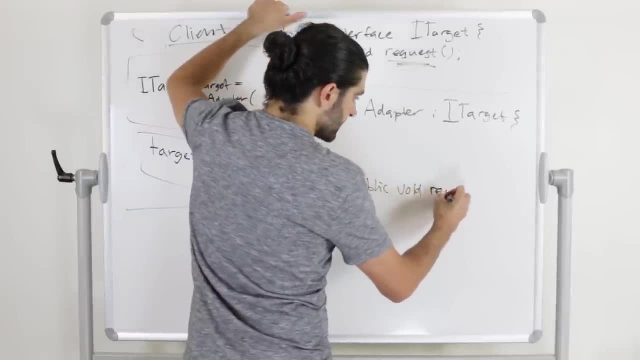 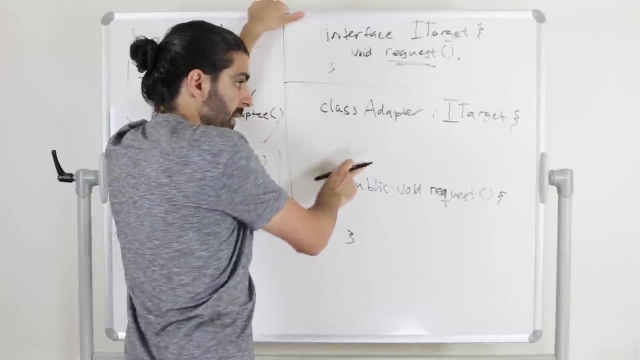 It returns nothing, So it's void And it's called request And it takes no arguments. And then it has some implementation. And what's the implementation here? This is the reason I left this white space. This implementation depends on our particular scenario And in this particular hypothetical example, we want to be able 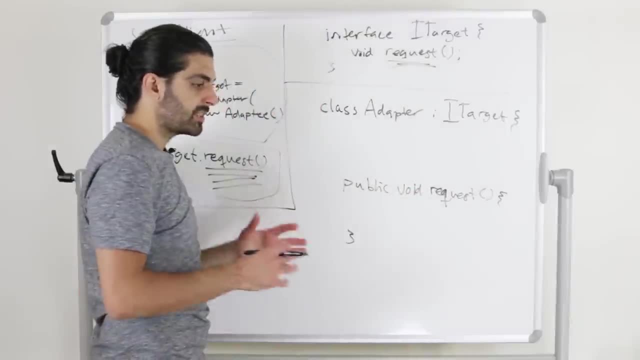 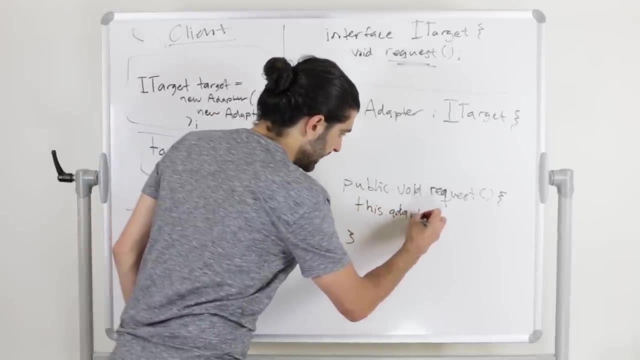 to use the constructor, So the request method of this adapter needs to delegate to the adaptee. So let's assume we have an adaptee which we can access by saying thisadaptee, And this adaptee has the other type of the method, Has the other signature for that method that we want to call. 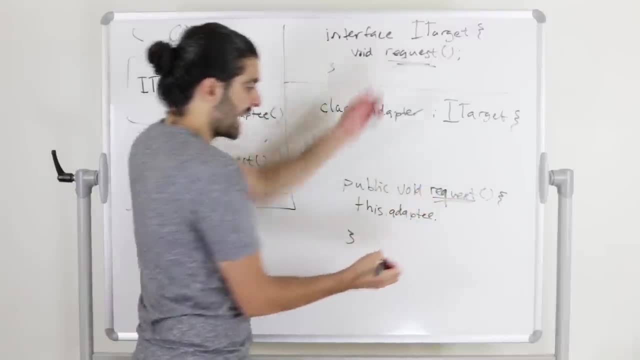 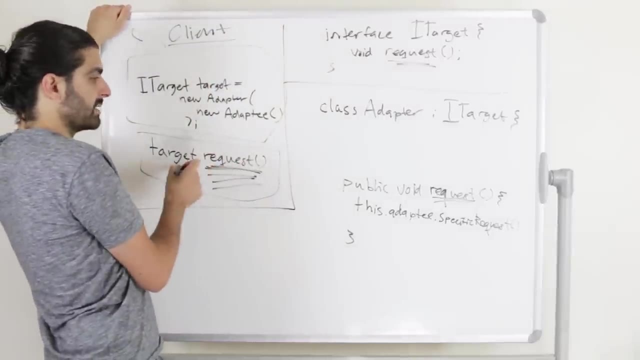 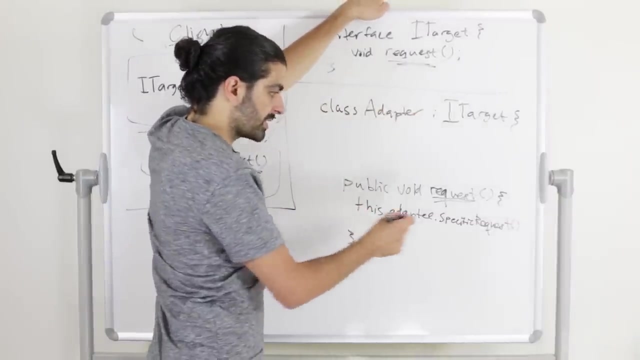 We now use the signature request But actually the adaptee has a method called specific request. So the client is calling the method request on the target, which is a concrete adapter of type itarget, And this concrete adapter calls the method specific request on the adaptee. 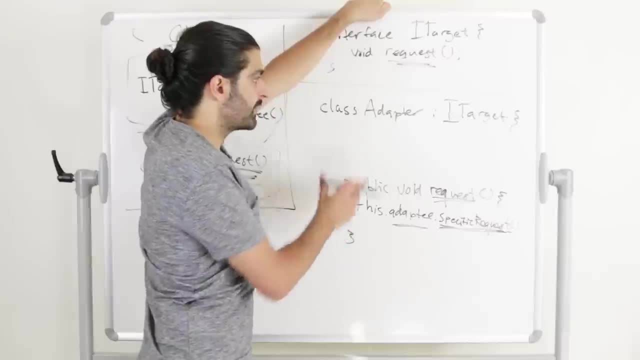 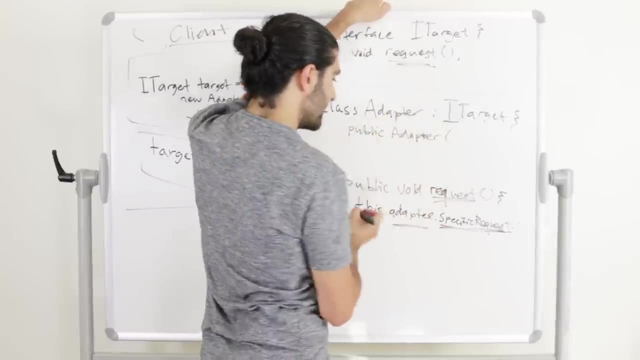 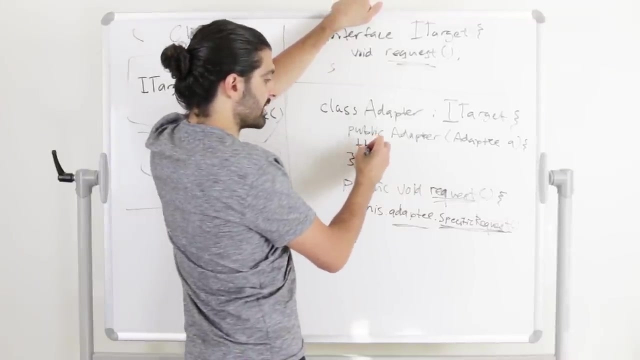 So the question, the only remaining question, is: how did the adaptee end up here in the adapter? Well, ask the constructor. Click adapter that takes something of type adaptee. To save space, I'll just name it a And then we'll set that to a private instance variable. Thisadaptee equals a. 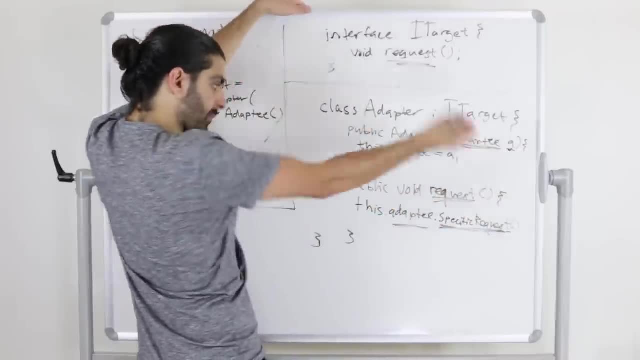 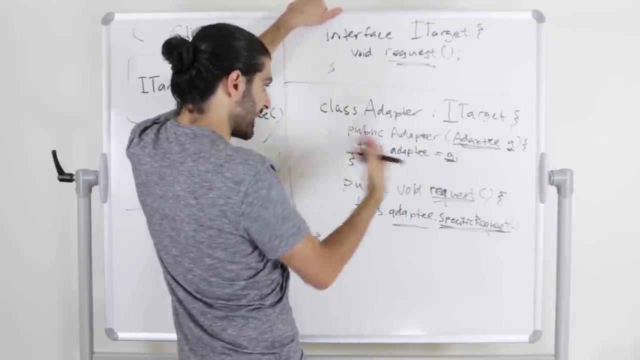 In other words, this adaptee called a that we passed through the constructor or that we are passed through the constructor. We take that a, we take that adaptee and we put it in, we assign it to the instance variable adaptee By saying: thisadaptee equals: 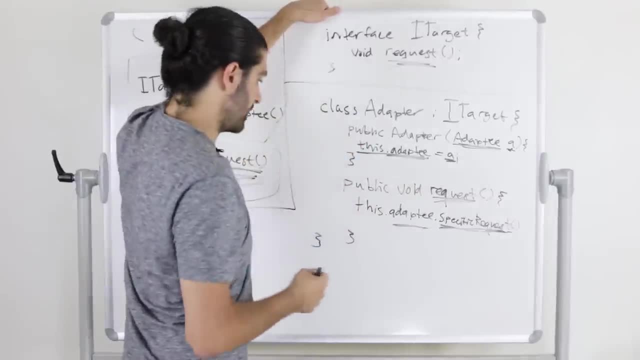 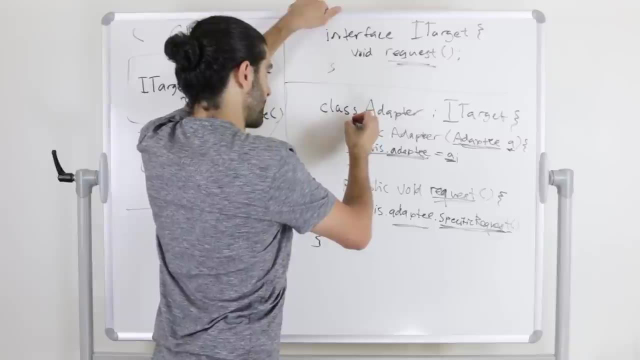 a And of course then we actually need this private member, this instance variable, which I always forget this. so now it becomes super crammed, but let's just put it here. So let's assume that private is implicit. so let's just say that we say there's an instance variable. 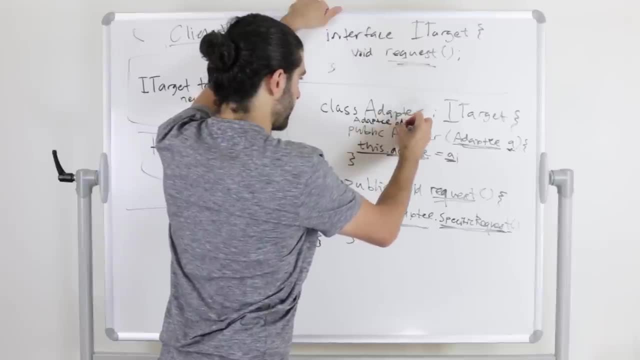 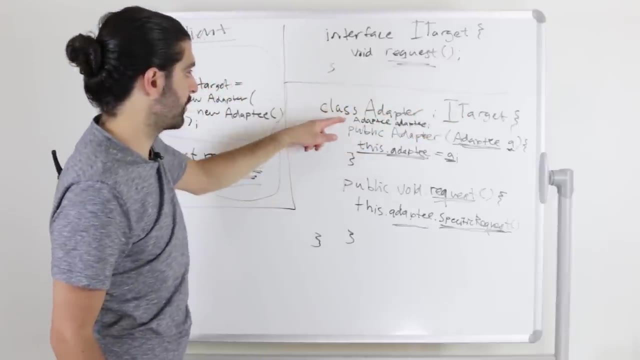 of type adaptee and it's called adaptee. So again, sorry about the space, but let's just recap. There's a class called adapter, It's of type itarget, It has a private instance variable called adaptee And when we run the constructor, the constructor needs to be. 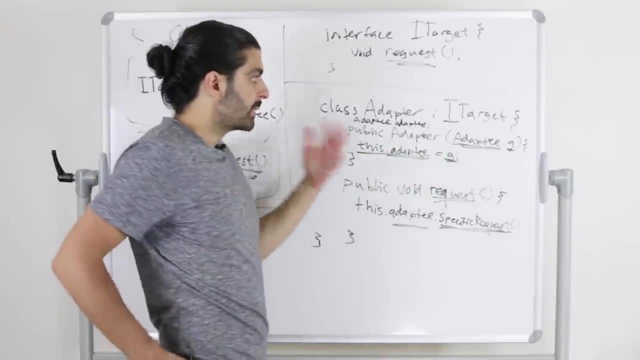 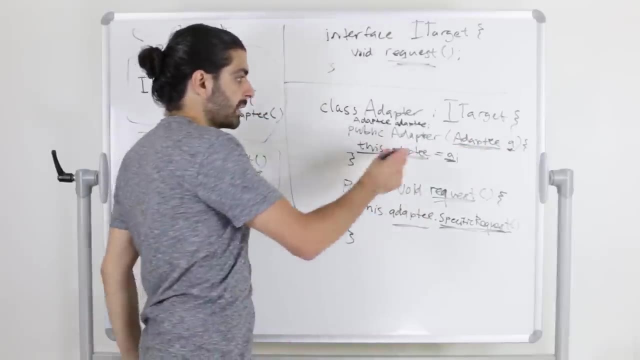 called with an argument. or rather, when instantiating the class, we need to construct it with an argument and that argument needs to be of type adaptee, And then we'll call that argument a, because here we'll set this private instance variable adaptee to this a that we were passed. 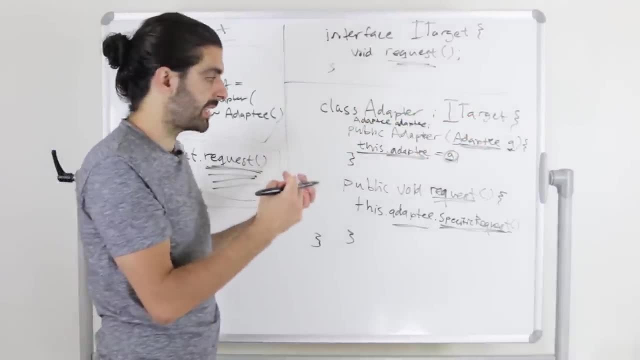 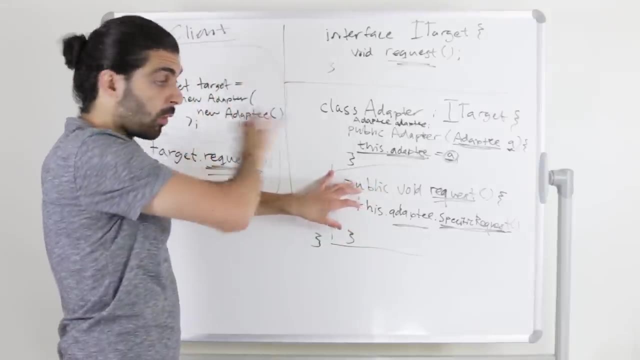 in. That's the constructor. So the constructor simply takes that adaptee and assigns it within the scope of this instance. Then we have the method request And request. is this method that we want to be able to call from the outside? It's public, it returns nothing and it's called. 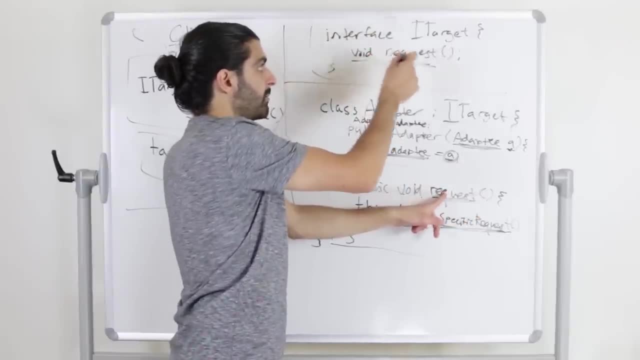 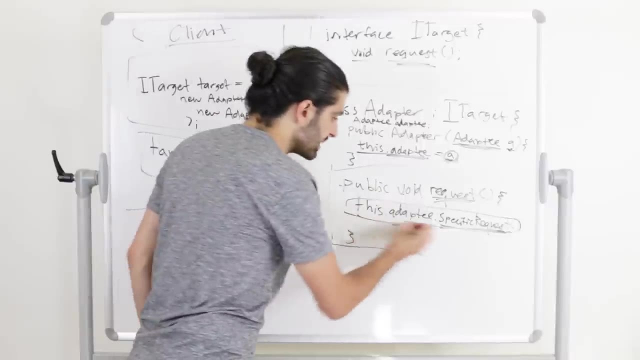 request, Because it follows this interface, where it has to be public and it has to be void and it has to be called request. It takes no arguments And what this method does is essentially this: It simply takes this adaptee that we just created, We created through the constructor. 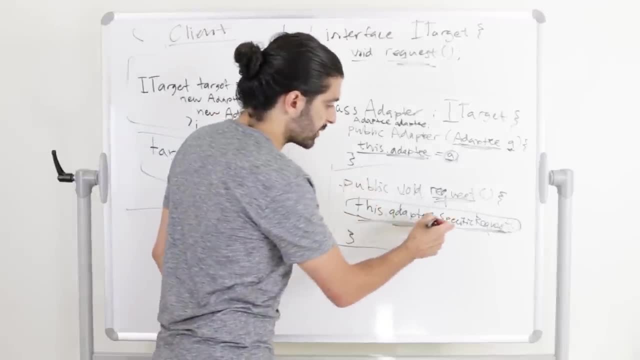 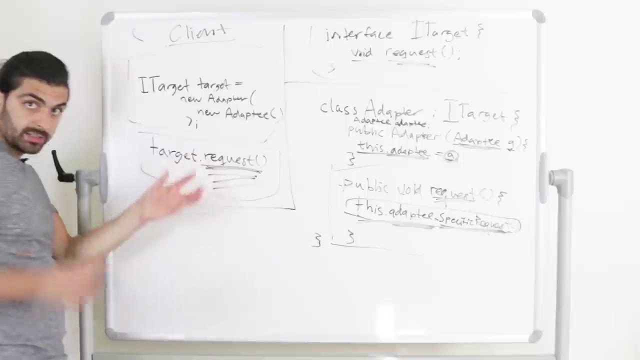 that we assigned to via the constructor. It takes that adaptee and it calls the method specific request. So we call the method request on the adapter, but eventually that means that we'll call the method specific request on the adaptee. And the only thing missing. 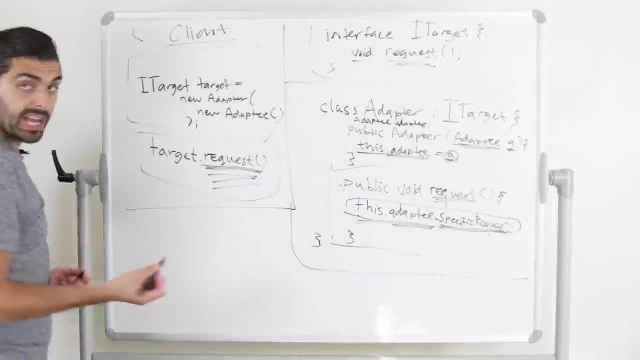 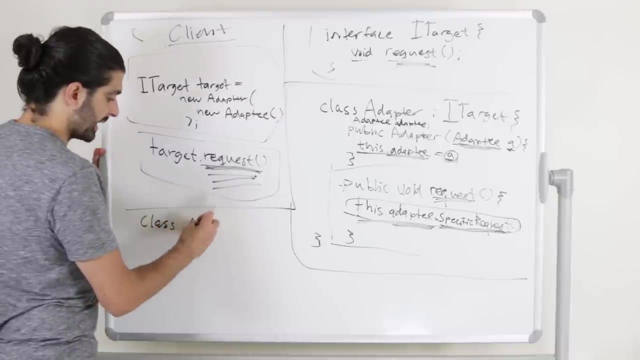 now is really the adaptee, But again, the adaptee could look like whatever. I mean, it depends on your scenario. But in this case, of course, we have the method specific request. so let's build that. So let's say that we have a class called adaptee and this is what 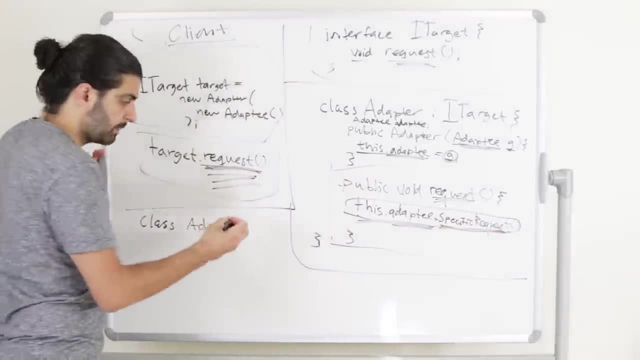 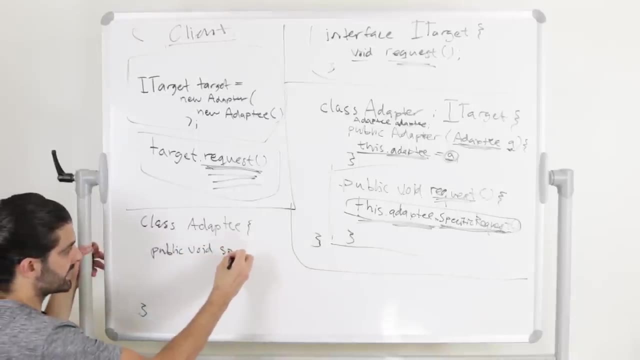 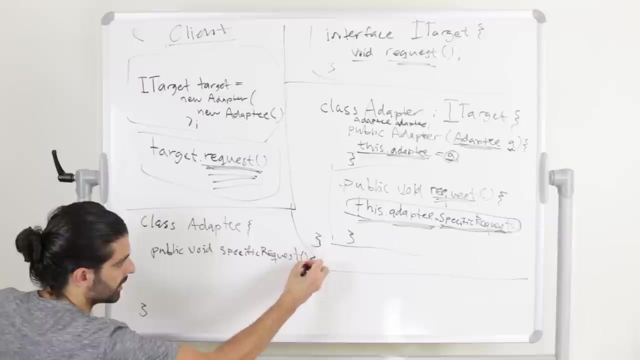 was in the rightmost corner in the picture we drew before, like in the UML, And this adaptee simply has an instance method, a public void method that is called specific request. Sorry about the space, as usual, Public void, specific request. it takes no arguments and 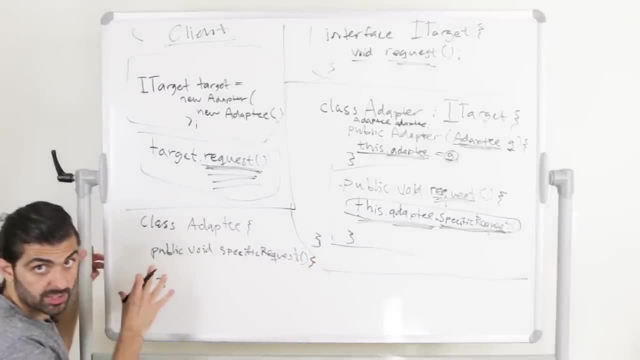 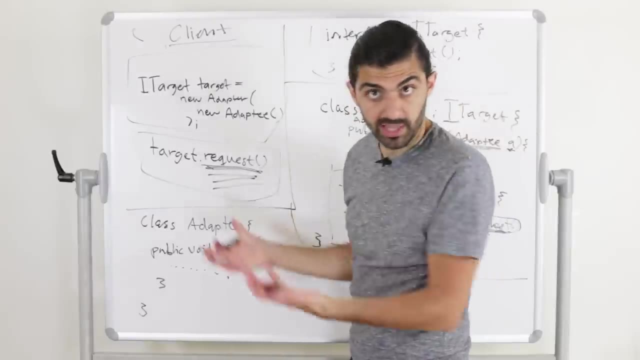 and it has some implementation, and whatever that implementation is is completely outside of the scope of this discussion, And so this ADAPT could be an external library. it could be something that you're trying to deprecate step by step. it's something that you wrote. 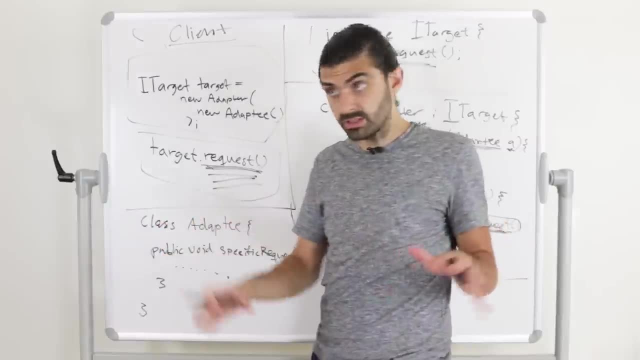 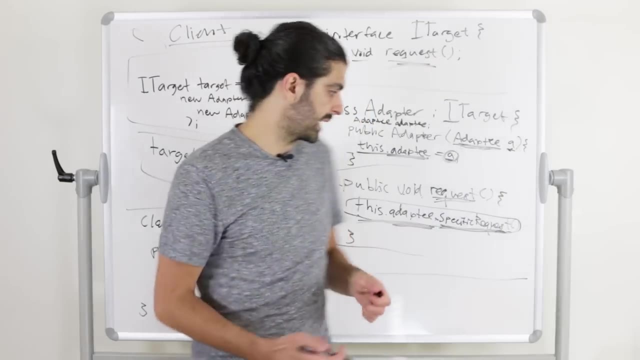 but that you want to get rid of, but you're not ready to get rid of in all the places at once. So you want to adapt it in particular places but use it with the old syntax in other places. So let's actually just think about that. 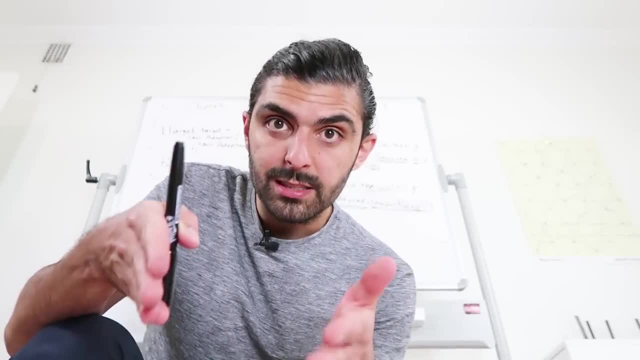 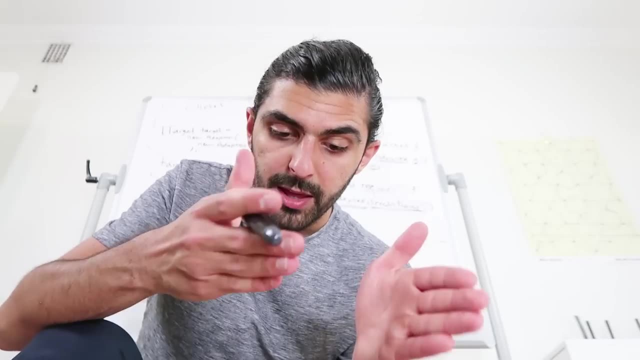 So, as a concrete example, I was looking at the documentation of the Nodejs library, Highland. I mean, this is just an example, you don't necessarily have to dig into the details- And in this documentation I noticed that the method reduce had one argument order. 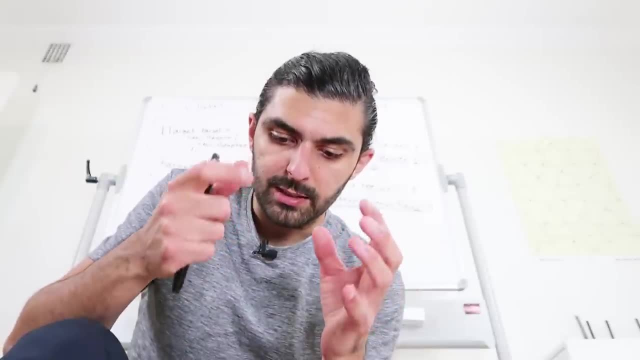 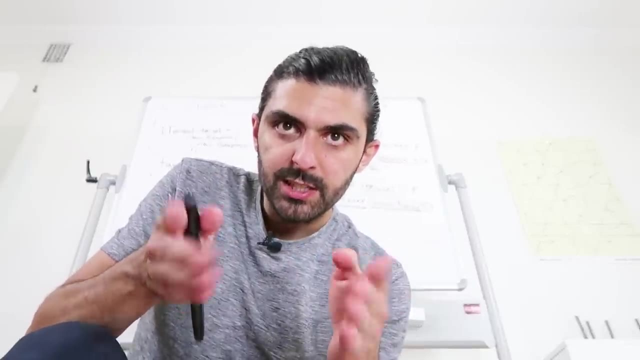 So the function reduce expect you to pass it two things and expected you to pass it in one particular order. But the interesting point is that in this documentation it said that in the next major release we'll flip the order of these arguments. So for some reason it was originally implemented. 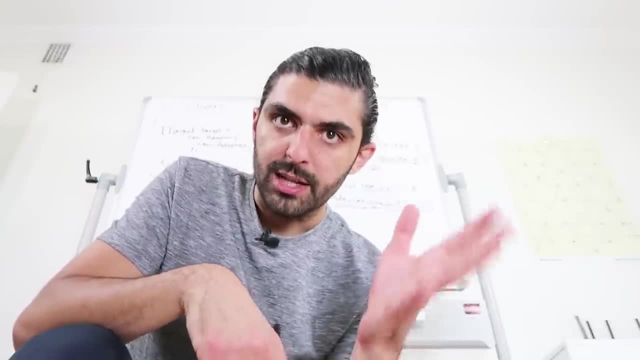 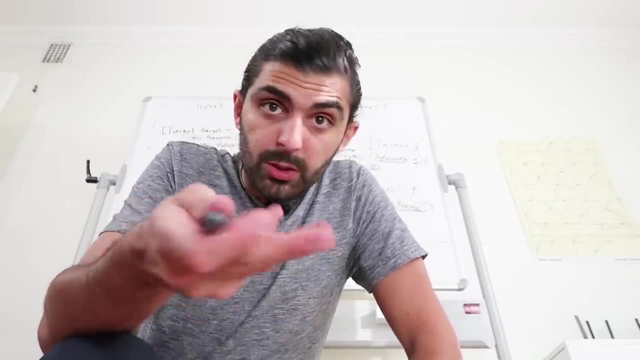 with one order of the arguments, And then around the road they realized that oh, actually it would be better if we would flip the order of the arguments and pass them in this other way instead. So one way of dealing with this could potentially be an adapter. 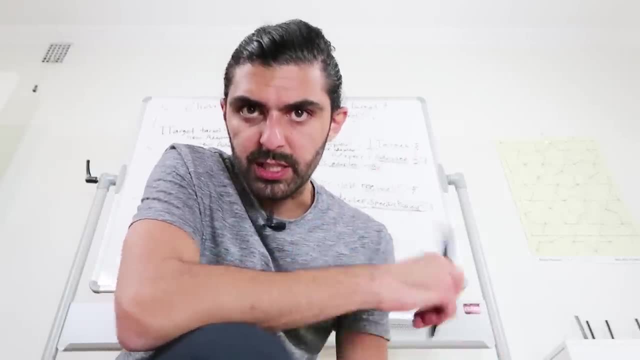 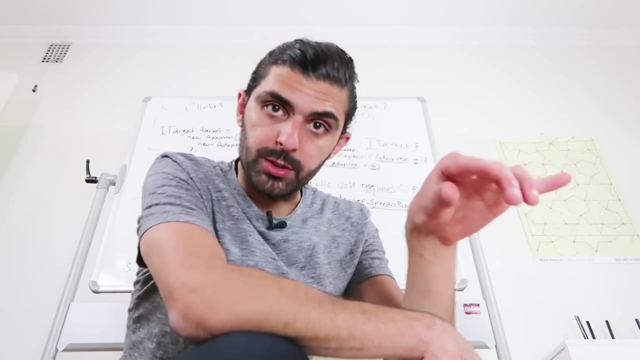 So, hypothetically, if you would want to use this new syntax or this new signature today, we could simply create an adapter and adapt one of the pieces. So you have argument order one and argument order two, and then you treat one as an adaptee. 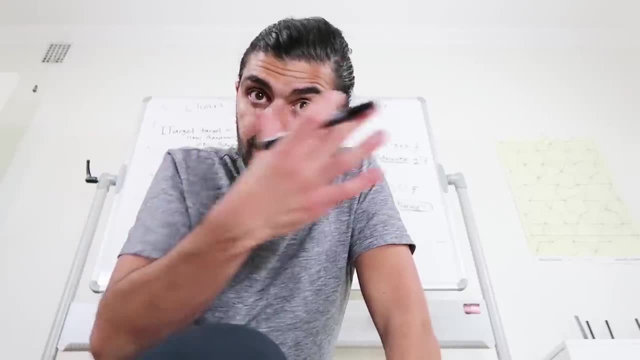 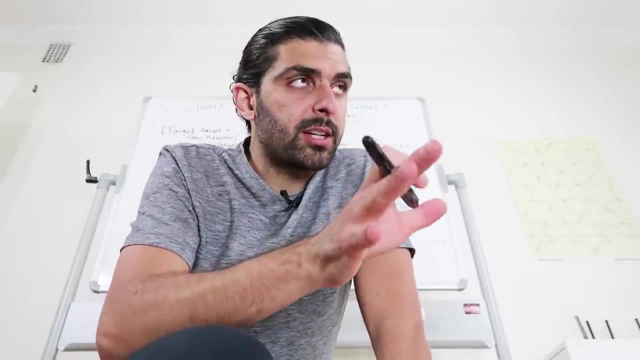 and the other as an adapter. So the adapter uses the other implementation Because, again, like point is that we just want to change the interface, We just want to change the order of the arguments. We don't actually want to re-implement the logic. 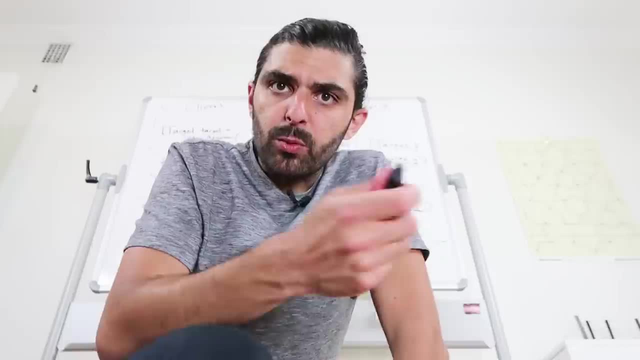 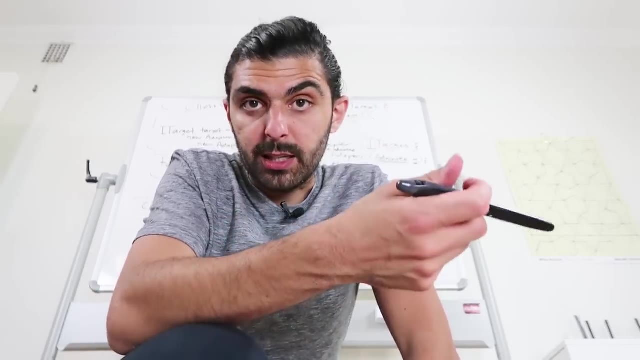 of that particular thing. So one just delegates to the other. Actually, think about the word indirection. This is introducing a level of indirection. Instead of calling the thing that we want to call directly, we call a thing that calls the thing. 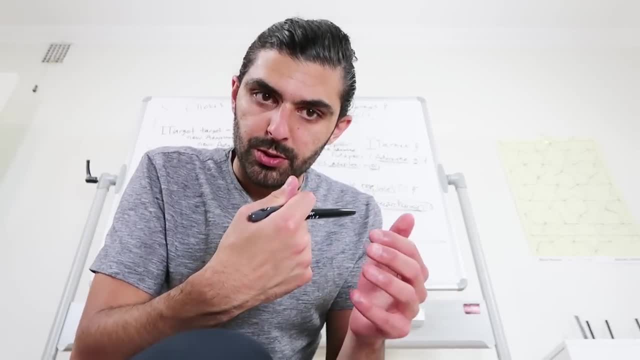 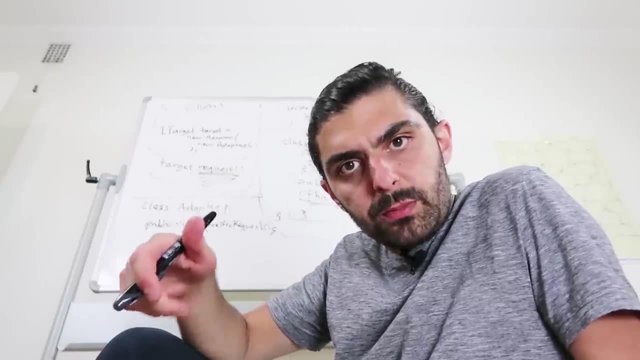 And this is what enables us to call the thing using one signature when it in actuality has a different signature. Another thing that I find interesting is the fact that we pass the adaptee through the constructor. Let's look at that. What we did here is that we pass the adaptee. 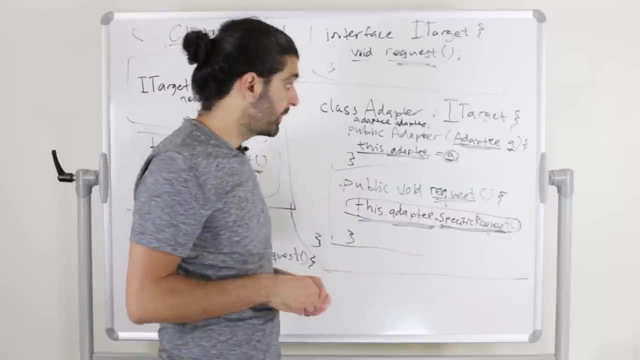 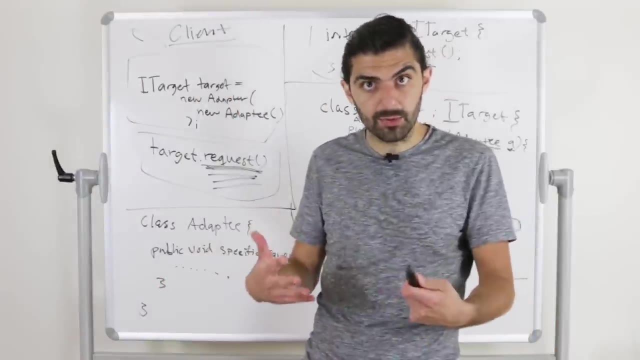 through the constructor. This is super good because it's dependency injection, but that assumes that the adaptee is instantiateable. So, going back to what we were saying before, if the adaptee is an external library and if that external library for some unfortunate reason, 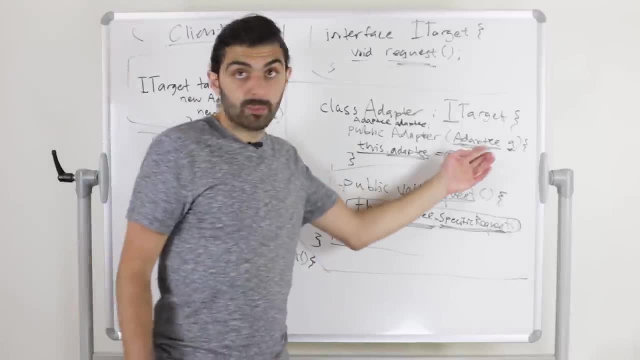 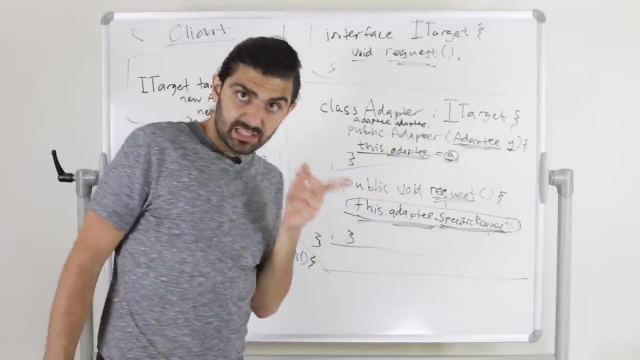 actually uses static methods rather than instance methods. we can't pass this adaptee Now. I would guess- but please correct me if I'm incorrect- that even if we didn't pass the adaptee, because the adaptee is static- we could still have an adapter. 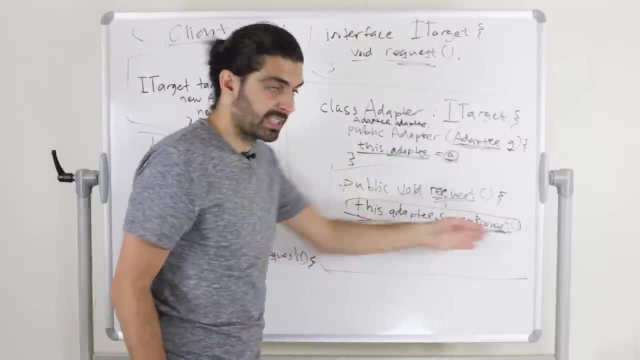 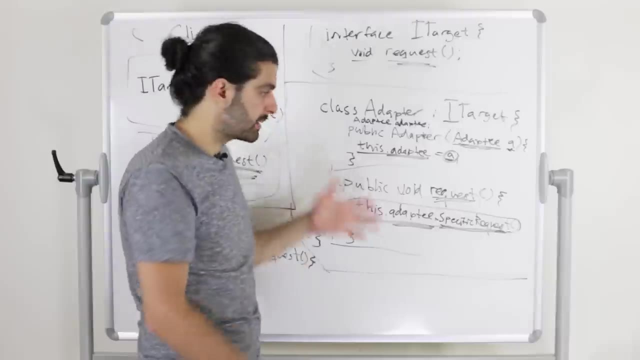 an adapter that adapts the request by calling the static method. So we still treat the adapter as an instance, because we're in object-oriented programming, So we should be using instances and not static methods, but we wouldn't say thisadapteespecificRequest. 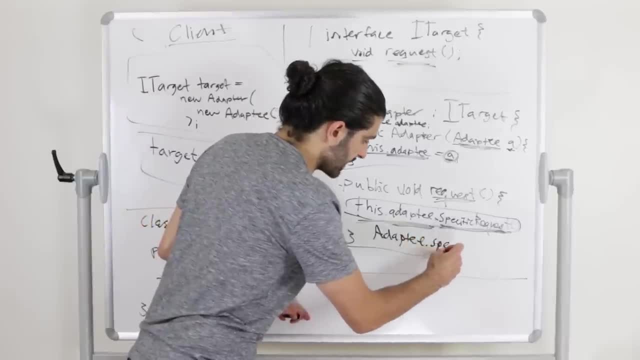 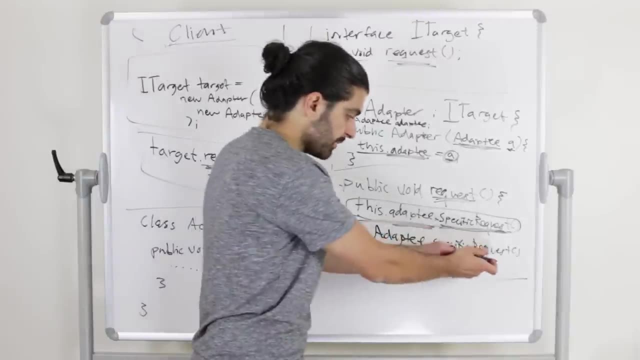 We would say adapteespecificRequest. Note that I used a capital A here to denote that we're statically accessing the class. So it's a class method. So we're calling specific request on the class adaptee and not on the instance adaptee. 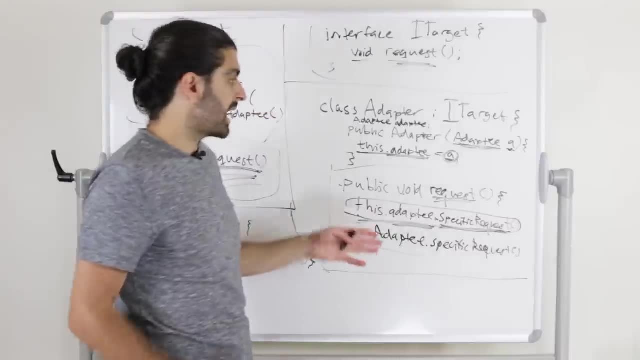 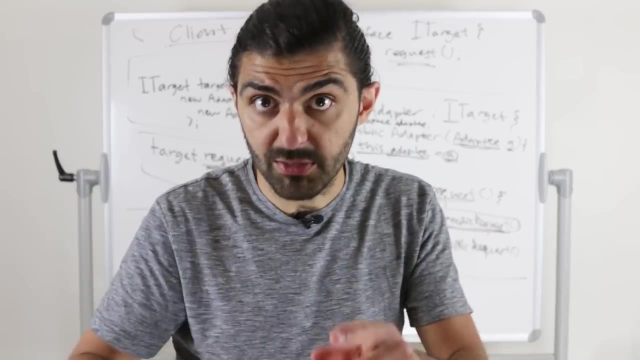 Hopefully, of course, our libraries use, but in this case I would still actually deem this an adapter pattern. Please correct me if I'm incorrect. So I was kind of struggling with coming up with better examples, but if you do have a better example of adapter pattern, 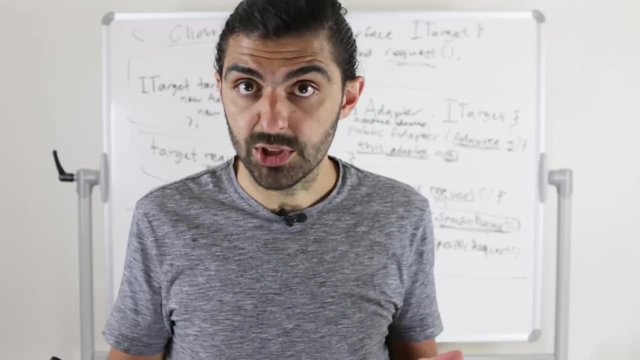 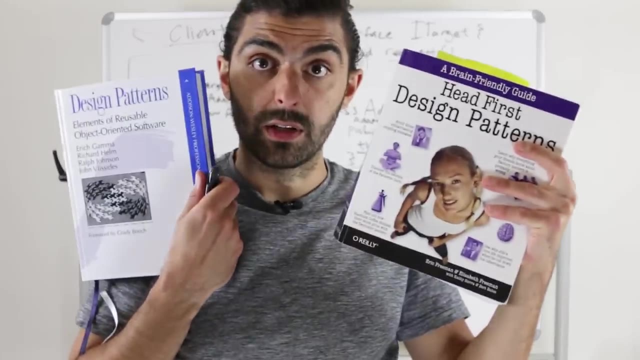 please do absolutely shoot that in the comments. I'm sure it would be massively appreciated by me and others. Now, before we wrap up, let me just mention one final thing In this book, and in this book they say that there are two versions of the adapter pattern. 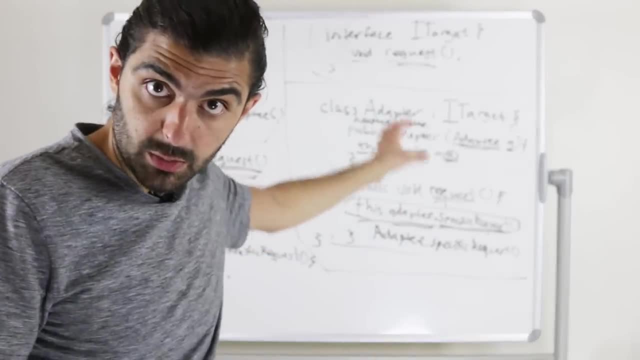 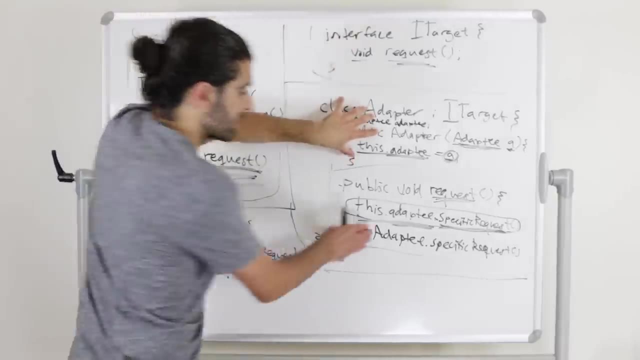 Super interesting One is this kind of composition way that we used it right Where you have a client that uses something of type iTarget and the concrete implementation of the iTarget. let's remove the static stuff. the concrete implementation of this target. 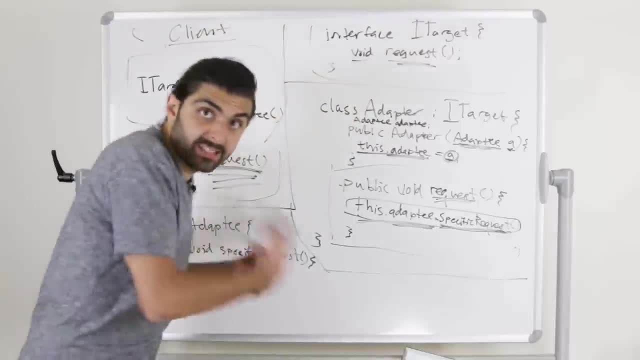 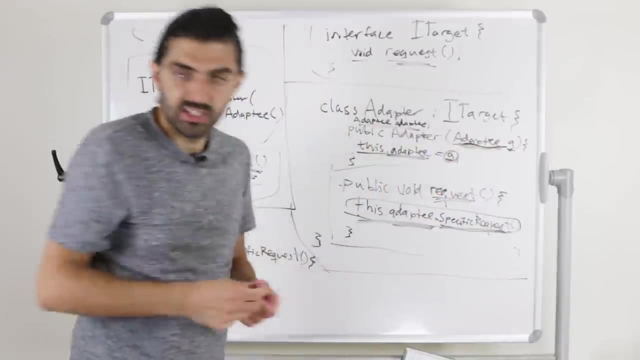 the adapter uses an adaptee, So it has an adaptee. The adapter gets an adaptee and has an adaptee and delegates to that adaptee, So it's by composition. The other way is through inheritance and not just any old inheritance. 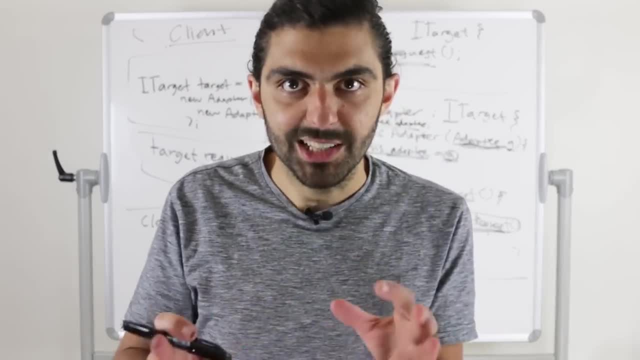 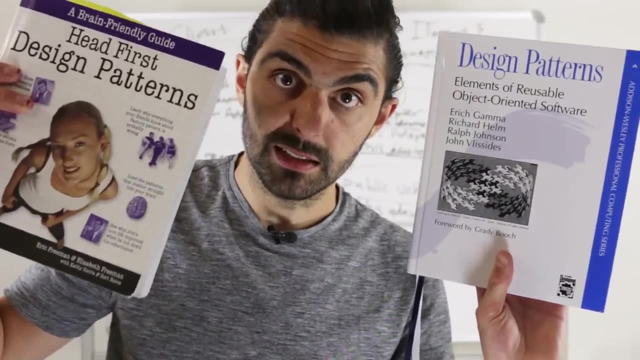 it's through multiple inheritance And that's the reason I'm not digging into that now, because I don't have enough experience with multiple inheritance. But if you find that intriguing, do absolutely get one of these books and have a further look into it. 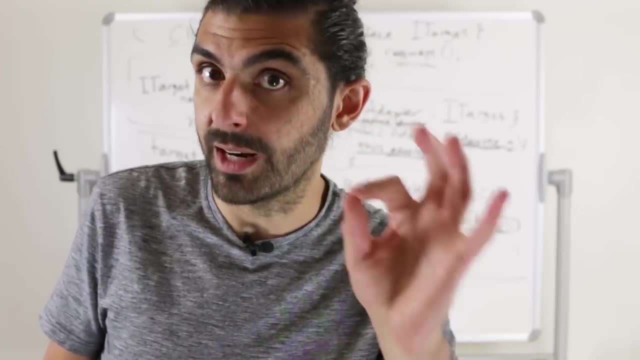 It seems that it's not too strange, but I kind of don't want to waste your time by going deep into something where I could be super wrong. But now you know there are two ways. This is one of the ways If you're in a language that doesn't support. 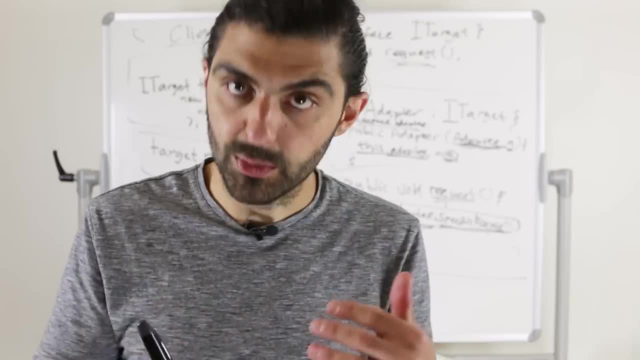 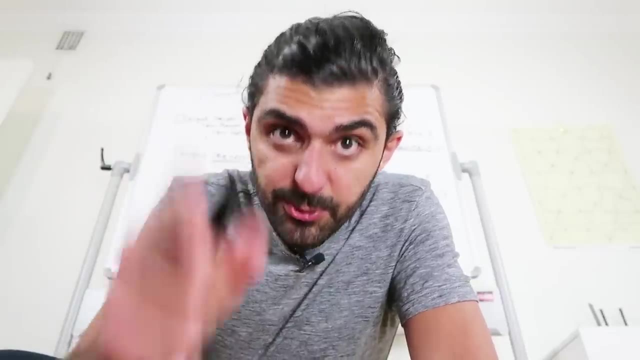 multiple inheritance. this is the way it's composition, But if you're in a language that does support multiple inheritance, there's another way and that might be the better way. So do have a look at that. So that's it for the adapter pattern.